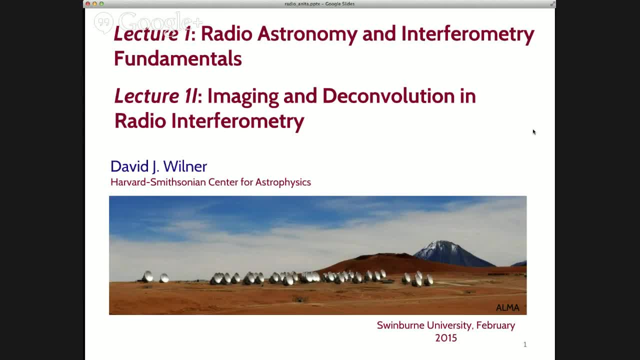 to hand it over to David now and he's going to give us the first lecture series. So this will be a general overview of radio astronomy and interferometry, and the second lecture will focus on more detailed discussion of imaging and deconvolution in radio interferometry. 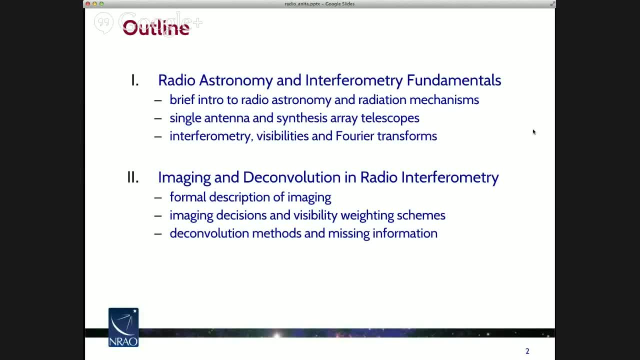 The outline of this first talk will be a brief introduction to radio astronomy and radiation mechanisms and radio wavelengths, Discussion of single wave wavelengths, Discussion of single antenna telescopes and synthesis array telescopes, And then a more in-depth discussion of interferometry visibilities and Fourier transforms. 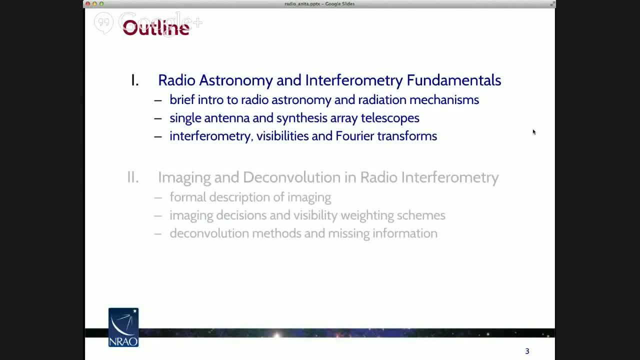 So this is the outline for today's lecture. My intent in these lectures is not to be entirely rigorous, but to give you a fundamental grounding in the most important concepts in these areas and also to allow you to develop some intuition about some of the more subtle aspects, particularly. 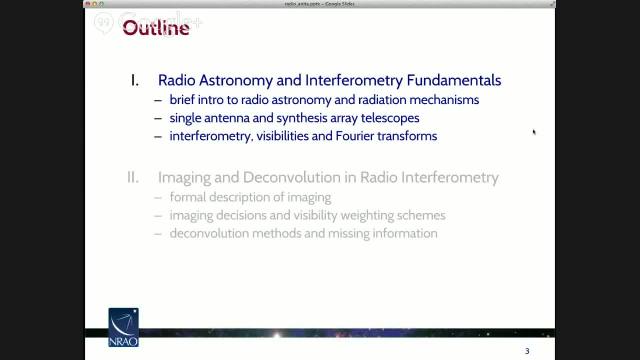 of interferometry. If you're looking for rigor, I'm going to give you a list of references where you can get as much rigor as you desire, So let's go into that just before we begin. I'd like to highly recommend Essential Radio. 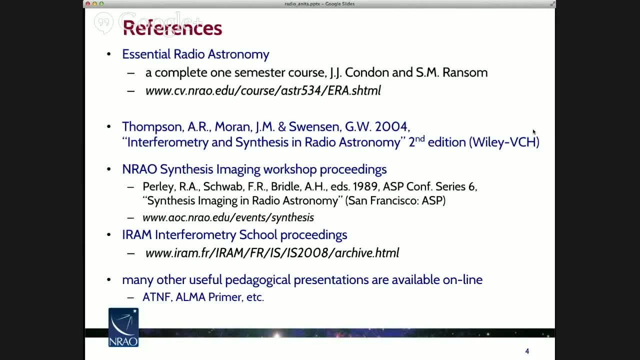 Astronomy. This is a complete one semester course developed by Jim Condon and Scott Ransom astronomy observatories in the us. all of the course notes are online. it's very detailed, very descriptive and and just a fantastic resource for interferometry. there's a reference: thompson moran. 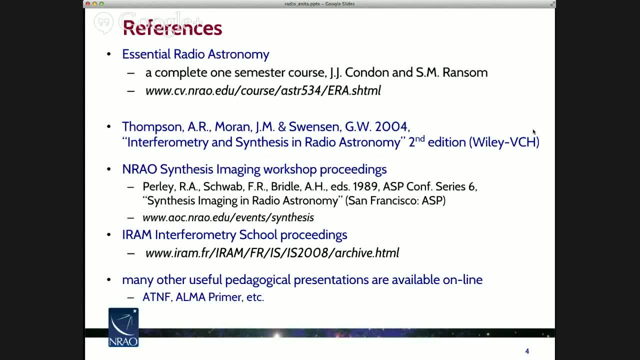 and swenson called interferometry and synthesis and radio astronomy. this is a difficult book to wade through, but if there's any topic that you're interested in and you need some fundamental derivation, it is surely in there, and so that is where you should go. for that rigor. there are also 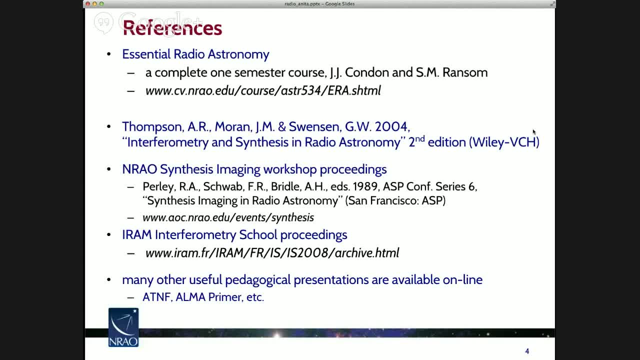 a wonderful summer school lectures available on the web, in particular the nrao synthesis imaging workshop proceedings and the iram interferometry school proceedings. some of my slides, in fact, are from my own lecture at the nrao synthesis workshop and you can go there and see see more about that. 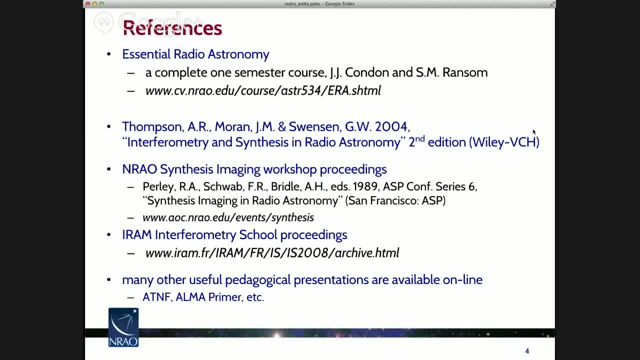 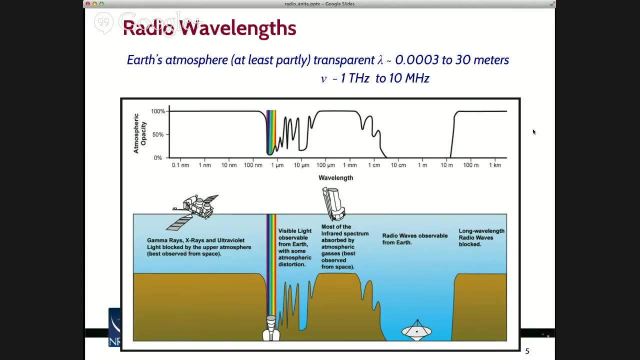 and you can find many other uh useful pedagogical uh presentations about these topics online: the atnf here in australia, um the alma primer and uh and many others. all right, so radio astronomy. what's special about radio wavelengths? well, i'm sure we're all familiar with the electromagnetic spectrum light described by its wavelength going from. 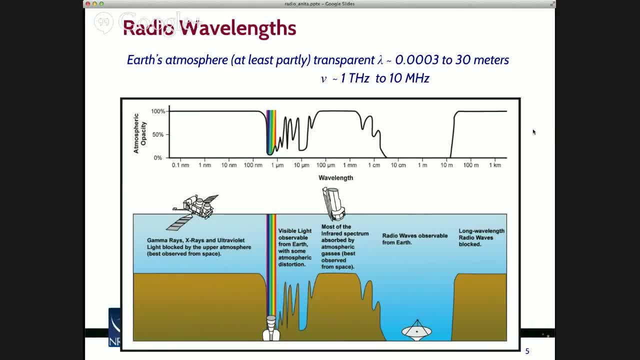 very short wavelengths: gamma rays, x-rays, ultraviolet, through the visible part of the spectrum to the infrared, the radio um and and the very longest radio waves. so radio wavelengths kind of loosely defined, are our wavelengths from a few hundred microns, um and beyond, out to many meters, or frequencies from a terahertz, um or uh or longer. and what's special? 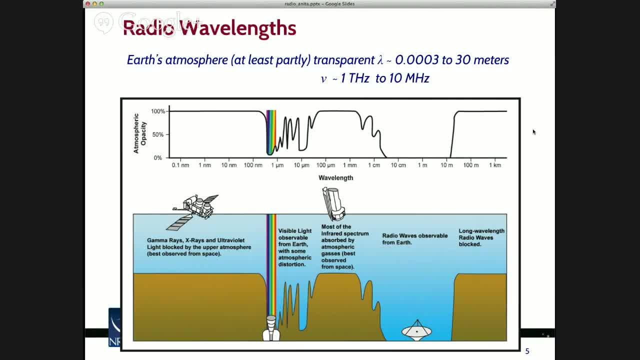 about radio wavelengths, as you can see in this chart, is that, like visible light, radio waves are almost always visible from the surface of the earth. so they're very important for radio astronomy because we can build large instruments on the surface of the earth to detect this electromagnetic radiation from cosmic sources. 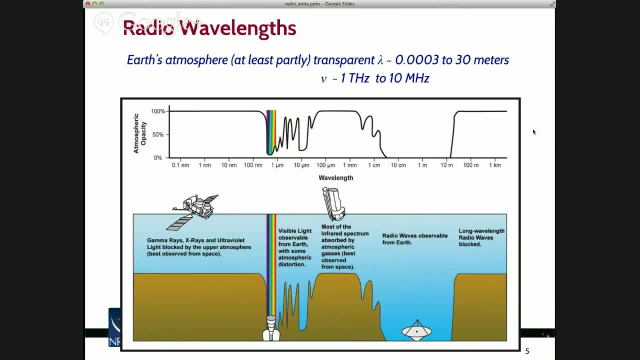 moreover, it's a very wide spectral window. it covers, you know, several decades in wavelength. it's much wider than the optical, in fact, and so there are a number of very important emission processes that come and go in various parts of the spectrum that i'll describe in a moment. a brief bit of history. like most aspects of astronomy, 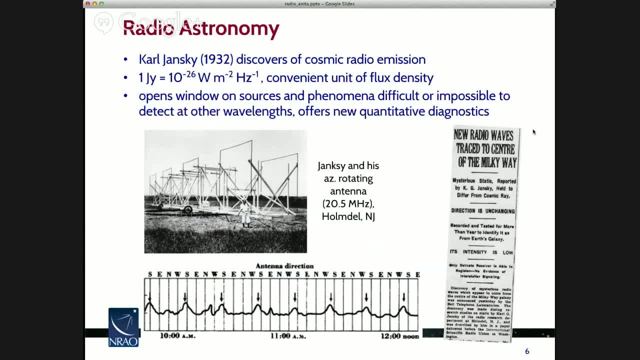 radio astronomy was a serendipitous discovery. carl jansky was employed by the bell telephone company and he was investigating, in the early 1930s, noise in short wave communications across the atlantic ocean and with his antenna pictured here in new jersey, he discovered. 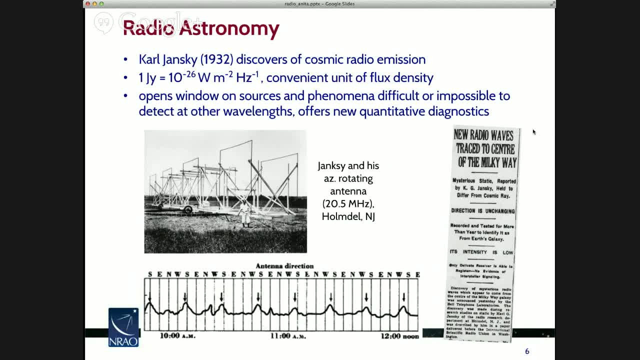 some noise and it was a periodic signal that he was able to locate with this rotating antenna to a specific part of the sky. he thought it might have something to do with the sun, but after discussing his discovery with an astronomer, he realized that the periodicity 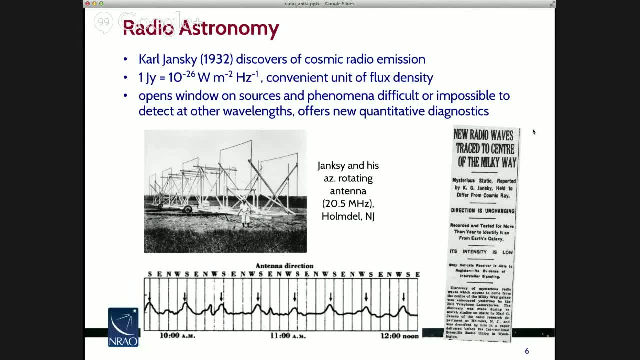 of his signal was not 24 hours, but 23 hours and 56 minutes, the sidereal rate. it was something that was actually fixed in the distant sky and not the sun, and it turned out to be the area of the galactic center, and this made headlines around the world. i have a little clip here: 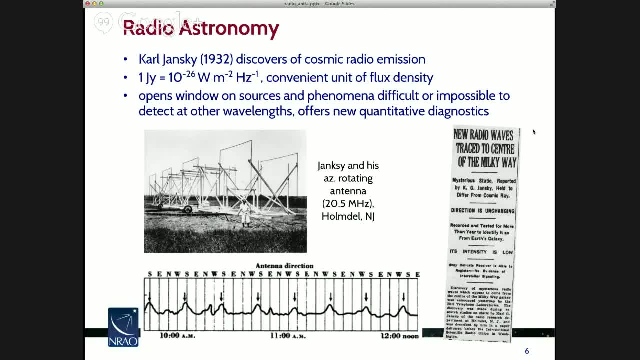 from the new york times. new radio waves traced to the center of the milky way. direction is unchanging and- my favorite comment- its intensity is low. that's something that radio astronomers have been dealing with ever since. jansky is immortalized with a unit of flux density. 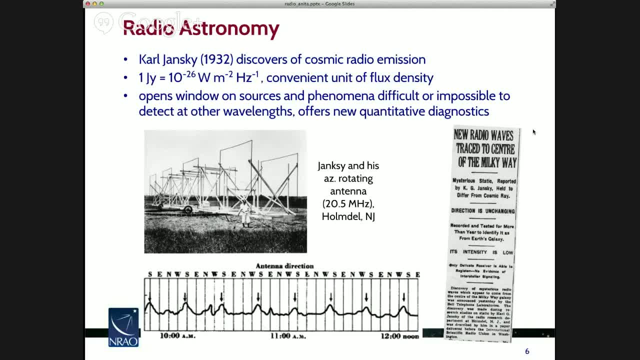 26 watts per square meter per hertz, and this discovery opened an entirely new window on on cosmic sources and phenomena that are either difficult or completely impossible to detect at any other wavelengths, and so a real new window on the universe. just as a postscript, this is all. 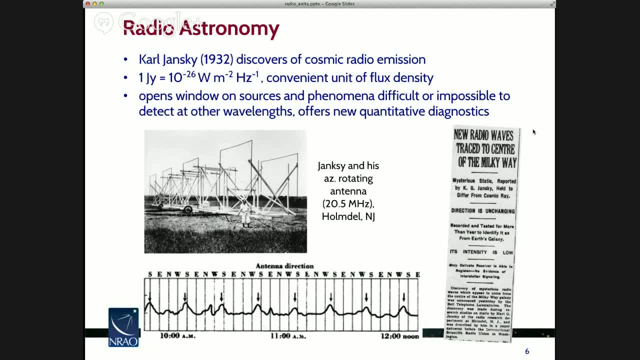 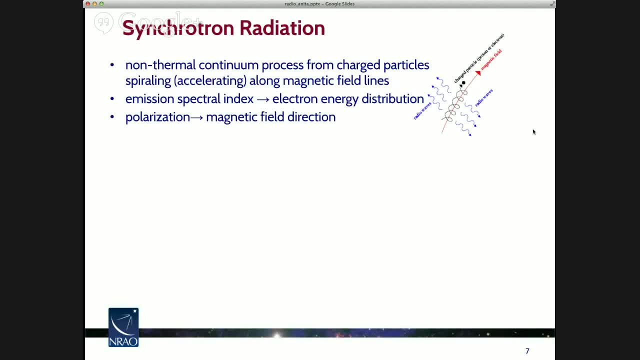 jansky did in radio astronomy. he was then assigned to other topics at bell labs and never returned to it. okay, so i'm going to go through a series of videos that are going to be useful for you to look at, and i'm going to go through a series of the most important emission mechanisms that we see. 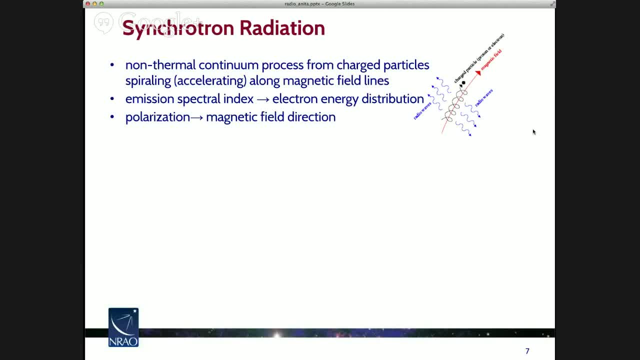 at radio wavelengths. one of the most important is synchrotron radiation. so this is a a continuum process from charged particles that spiral along magnetic field lines. so say, when an electron is spiraling along a magnetic field line it accelerates. that creates electromagnetic radiation from maxwell's equations and this radiation tells you something about the plasma. 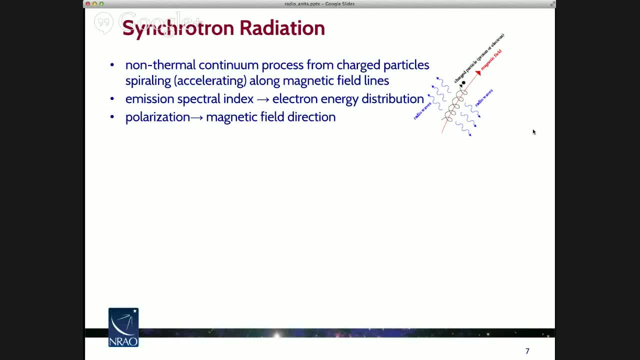 index, that is, the variation of the strength of the emission with frequency. can tell you something about the distribution of the electron energies and the polarization properties of the radiation? can tell you something about the magnetic field direction, because there's a preferred direction of the electrons spiraling. unfortunately, it looks like we lost the beautiful picture of cygnus a. 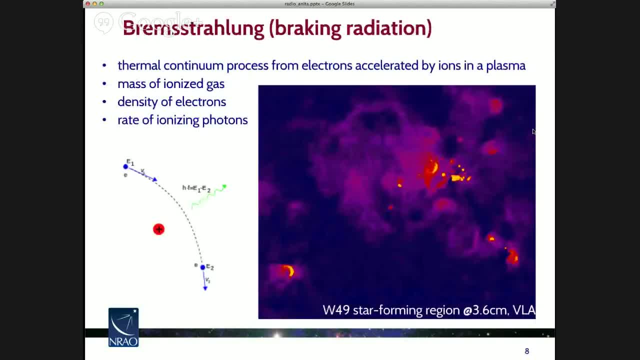 on this slide, which is too bad. okay, let's go on to the next radiation mechanism: bremstrong or breaking radiation. this is another continuum process from electrons accelerated in a plasma. only this case the electrons are are encountering protons and they're they're being braked, and so that acceleration creates. 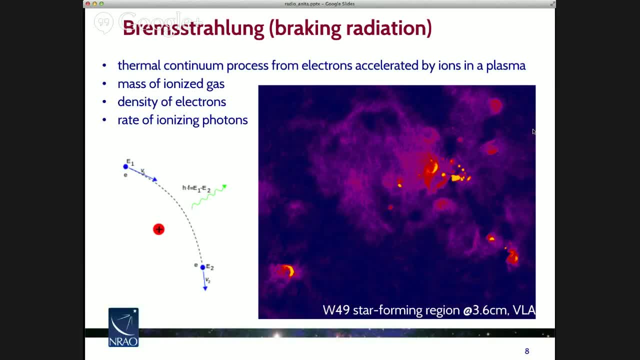 some electromagnetic radiation. this beautiful picture here is a star forming region at 3.6 centimeters wavelength, with a very large array of these little peaks. here are sources of plasma ionized gas which are being ionized by an embedded hot star which has enough ultraviolet radiation to knock the electrons off the protons. 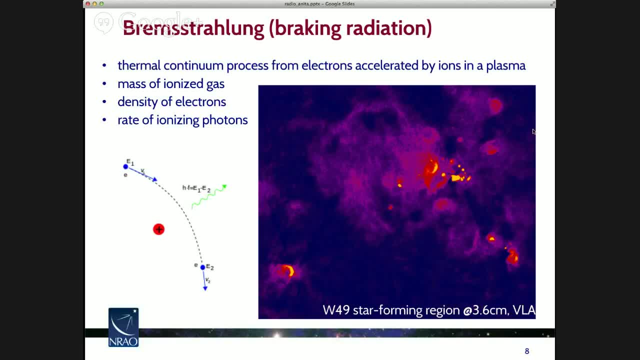 and from the intensity of this, of this emission, you can determine the mass of the ionized gas, the density of the electrons and indeed the rate of the ionizing photons. so something about the embedded stars which are completely invisible at really any other wavelength. another very important process, particularly at the shorter 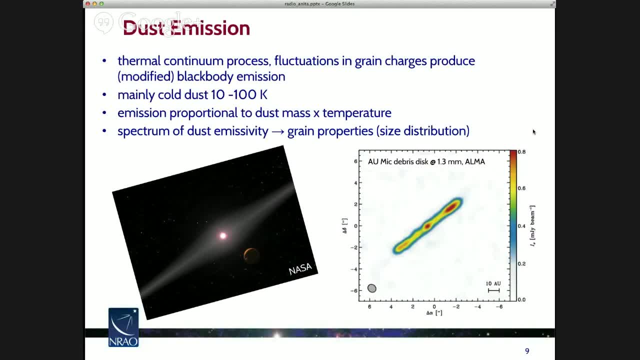 way your wavelengths is dust emission, another continuum process where fluctuations in the charges on grains produce essentially a form of thermal emission, a modified black body. this is most important in the radio, for coal dust tends to 100 kelvin and in this case the emission is proportional to the dust mass times, the temperature of the ionized gas, which is 10. 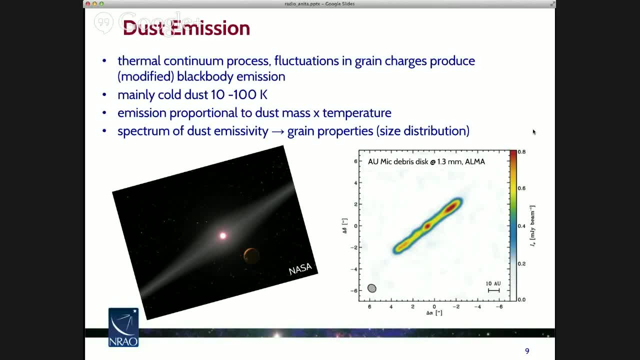 times the temperature of the dust. so one can learn something about the properties of the material and the spectrum of the dust emissivity. the change as a function of wavelength can tell you something about the grain properties, in particular the distribution of the grain sizes. here on the right is a recent image of dust emission from an edge on disk around a nearby star. 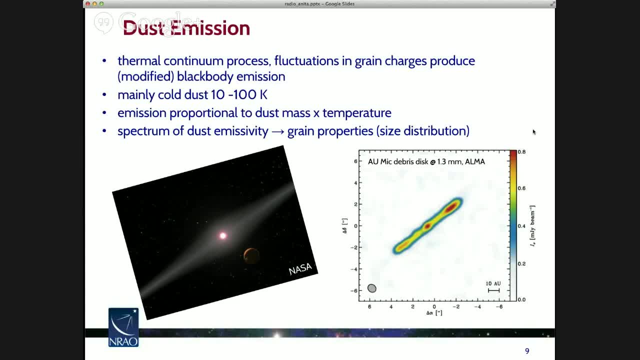 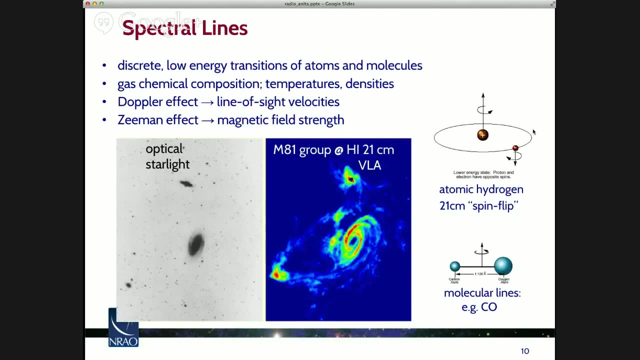 this is sort of a kuiper belt around the star au microscopy. so there's a lot of more things going on here, though yet further away than this, but a lot of studies are going on here as well, to start with this example, which is a blinding technology that produces about 1 to 10 millimeter dust emission. 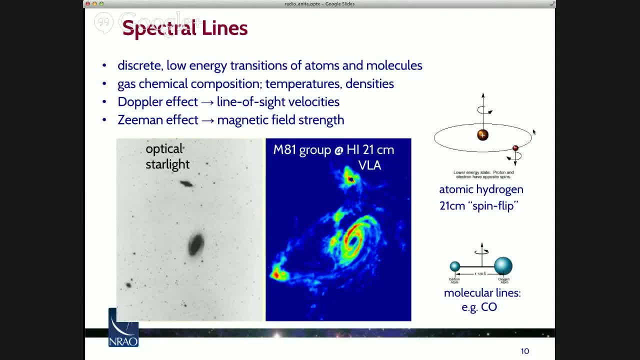 and the left is a nasa artist conception of what the system looks like. all right, equally, if not more important than these continuum emission processes that i've discussed, our emission from spectral lines. so these are discrete And that are observed. I have illustrated on the right one is the atomic hydrogen spin-flip transition at 21 centimeters, very famous. 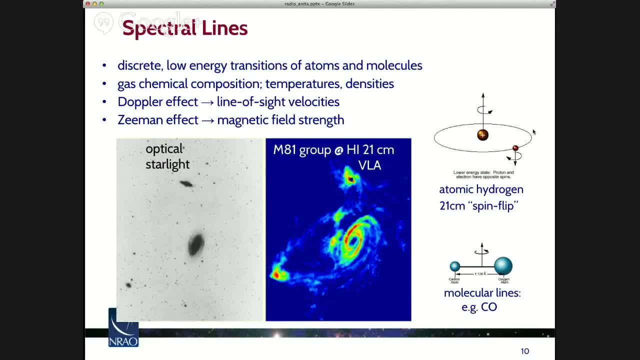 You can see in this side-by-side comparison of the M81 group that in the optical one can see the two galaxies very nicely, But that in the radio, in this 21 centimeter line which is showing you the neutral hydrogen, the galaxies show these incredible tidal tails and you can trace back how they've interacted in the future. 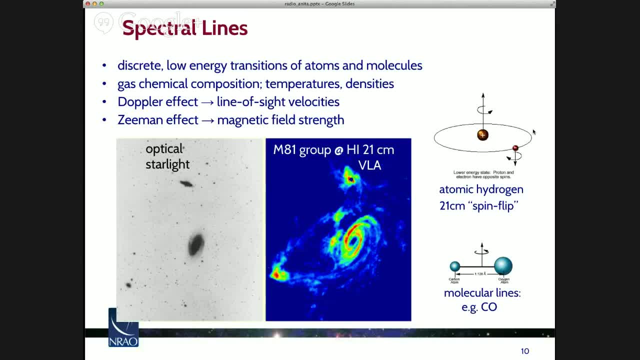 which is very difficult, if not impossible, to do from optical starlight alone. A second spectral line that's very important is the molecular line of carbon monoxide, CO. CO is found in regions with molecular hydrogen. Molecular hydrogen, when it's cold, has no spectral lines that emit. 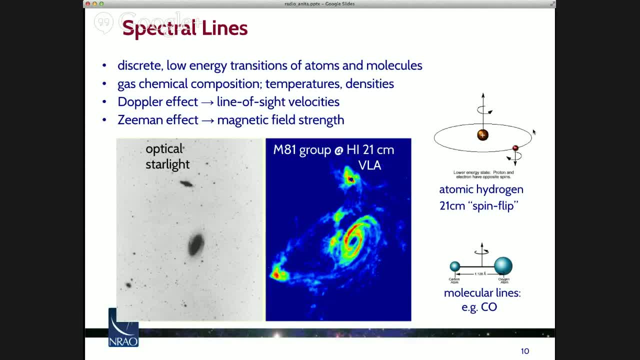 So it's very difficult to see. But collisions with the molecular hydrogen and CO excite the CO line, and so it's a way to trace regions of interstellar media that are molecular, And so with probes like this one can measure things like the gas-chemical composition. 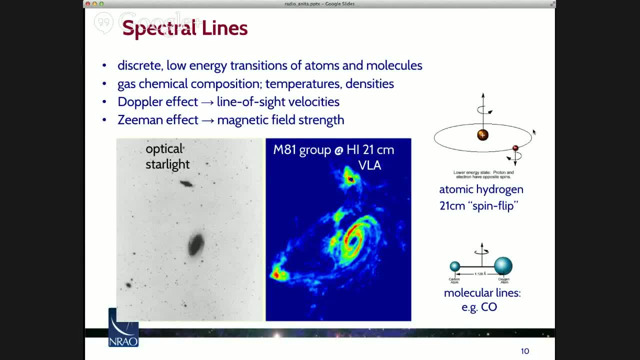 from different transitions of atoms and molecules get at temperatures and densities and other physical properties Extremely important. one can measure the Doppler shift of these discrete transitions, which gives information about light, Line of sight, velocities and kinematics. So one actually has a three-dimensional view of the M81 group. 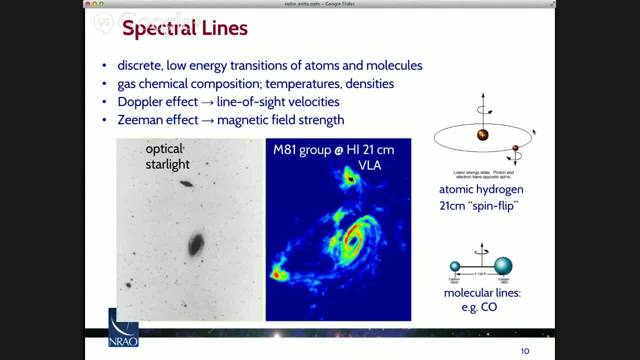 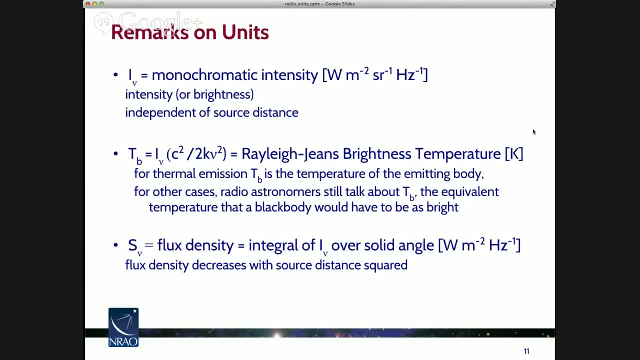 in the sense that there's another dimension of velocity here, And for some particular transitions one can measure the Zeeman effect, which gives information on the magnetic field strength, Another physical property that's very difficult to get at any other way. All right, 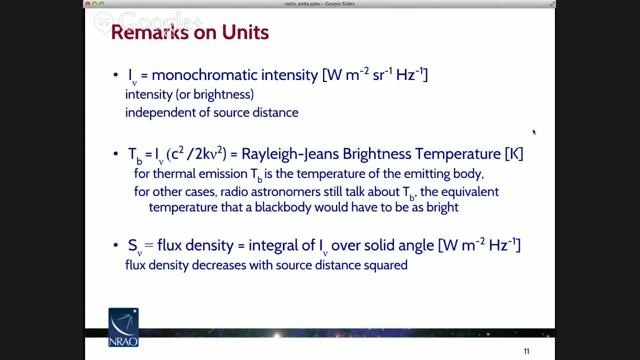 I'll make a quick remark on units in radio astronomy, because I have found in my experience that people find this very confusing. Intensity is an often-used unit, Quantity I mean, And its units are watts per square meter energy per steradian, per hertz. 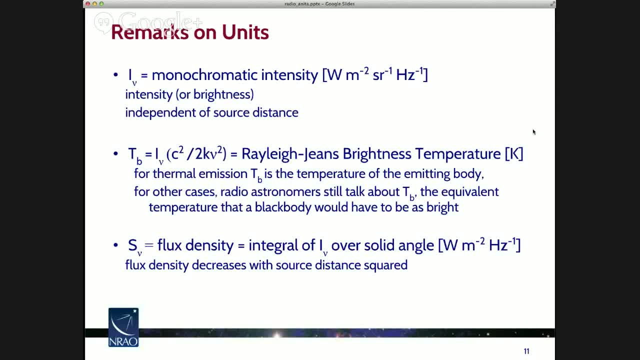 So this intensity is effectively a brightness and it's independent of source distance. So if you imagine looking at, say, the surface of the sun, if you resolve a little piece of that surface, it has some kind of intensity, And that's true no matter how far away it is. 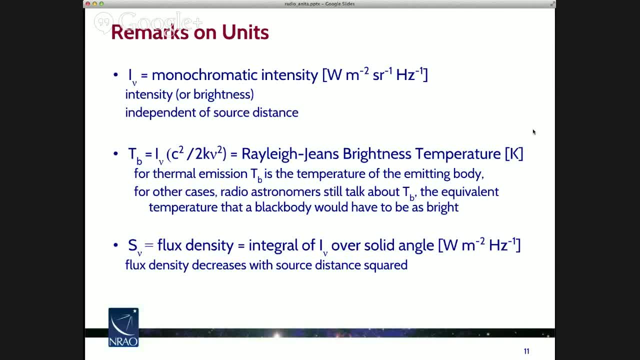 It may be 5,800 degrees, no matter how far away it is. Radio astronomers use a kind of peculiar unit called Raleigh-Jeans brightness temperature, which converts the intensity into a temperature, using the Raleigh-Jeans approximation. And so, for thermal emission processes, 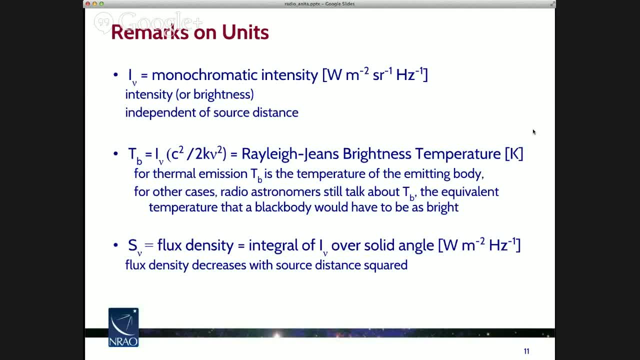 this brightness temperature is just the temperature of the emitting body, So we were looking at dust emission before. It might have a temperature of 10K or something like that For other cases, in particular all of those non-thermal processes I mentioned. 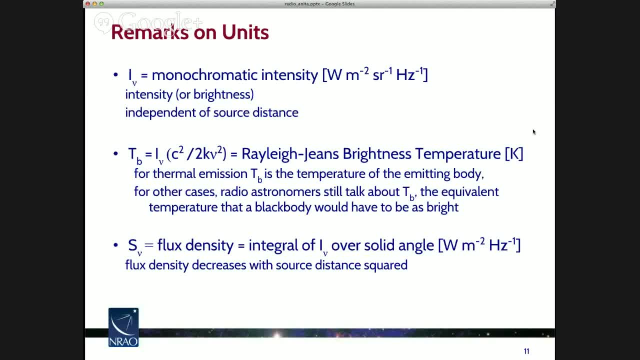 like synchrotron emission, radio astronomers still talk about brightness temperature, which you can determine with this formula. That's the temperature a black body would need to have to be that bright, but it doesn't correspond to any physical temperature, So that can be confusing. 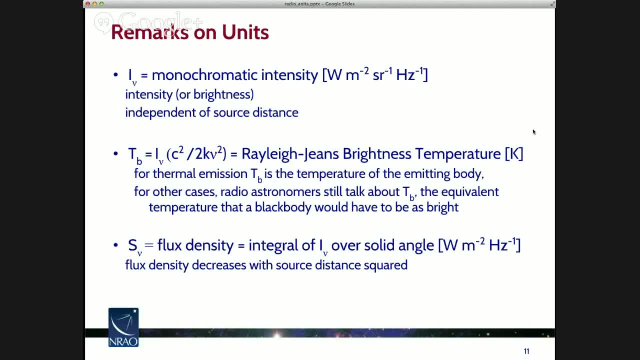 And then, finally, the most important unit is probably flux density, And this is just the integral of intensity over some solid angle. So flux density decreases with source distance squared, just as solid angle does. Okay, So if you're worried about units and you get confused, 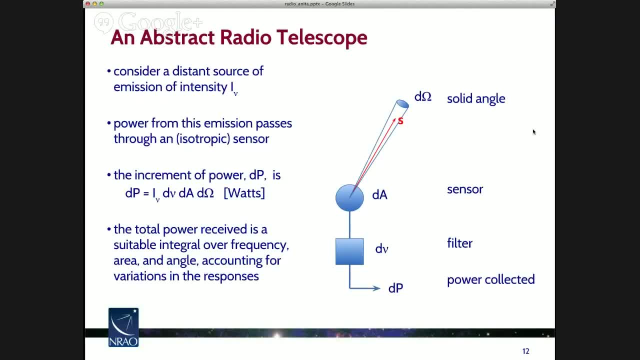 you might refer back to this slide. All right. What about a radio telescope? So this is a very abstract view of a radio telescope On this slide and I'll come to a more concrete example in a moment. but if you just consider a distance source of emission, 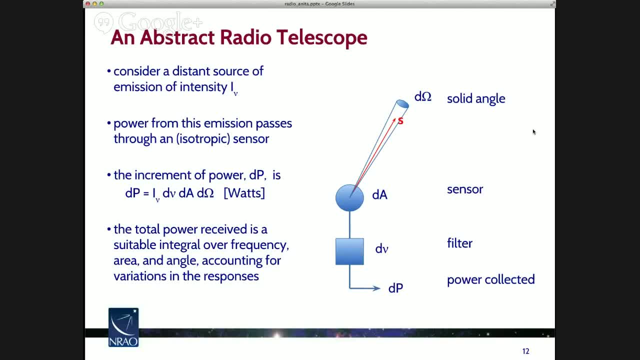 which has some intensity, I in some direction. then the power from this emission passes through some kind of sensor, some radio sensor, and that will increment power in the sensor. It's the intensity times, some differential frequency and area and solid angle, so power in watts. 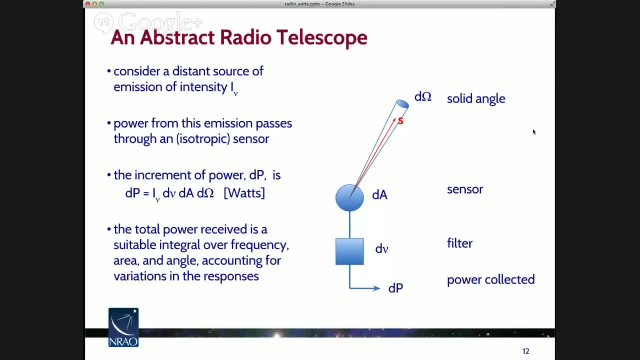 And so the power that you collect from the intensity of this distance source is a suitable integral right over these quantities of frequency, area and angle. And if you want to understand what that is, then for your telescope, of course, you have to understand what the response of the telescope is. 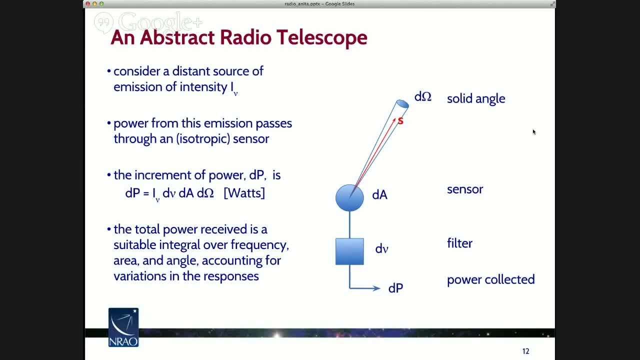 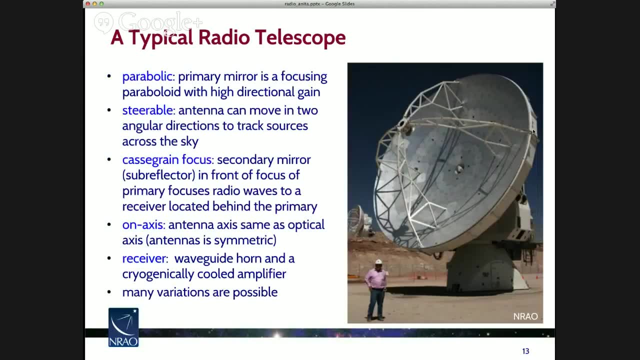 in all of these areas, how much collecting area it has, what the shape of the frequency sensitivity is, and whatnot. So here's a real radio telescope, a very typical one. This one kind of looks like an optical telescope in a way. 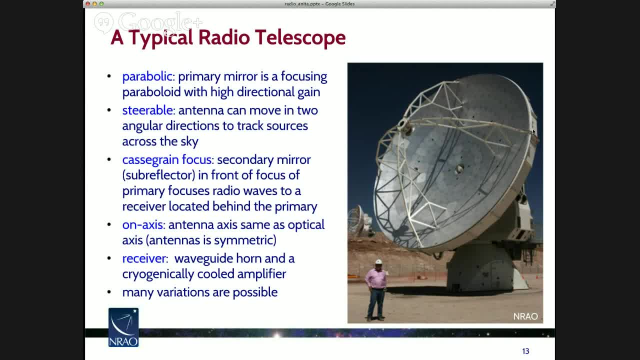 It has a parabolic primary mirror and that is a focusing paraboloid with high gain in some direction that collects all the radio waves and sends them to a focus. It's steerable, so it can move in two directions and track sources across the sky. 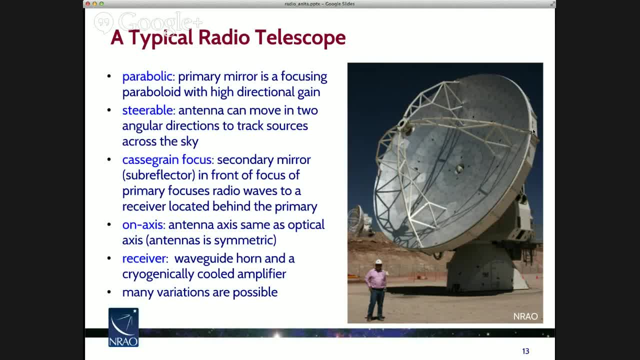 It has a secondary mirror, which in radio astronomy is often called a subreflector, which is in front of the focus and it sends the radio waves through the hole in the middle of the dish to a receiver that's located behind the primary. 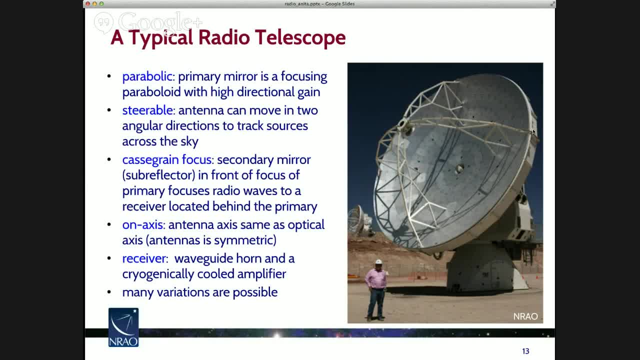 typically in a spacious, a relatively spacious cabin where one can put a lot of equipment. This particular telescope, you can see, is on axis, in the sense that the antenna axis is the same as the optical axis. It's symmetric. It need not be that way. 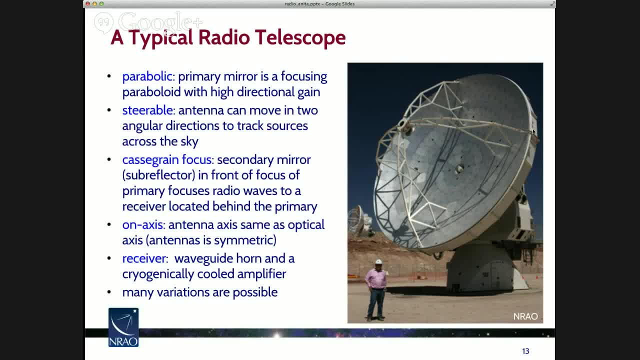 And the receiver in the back of this telescope is a little wave guide horn. that is just a little piece of metal which effectively collects the electromagnetic radiation and sends it to an amplifier which, in this case, is cryogenically cooled so that it reduces any background noise. 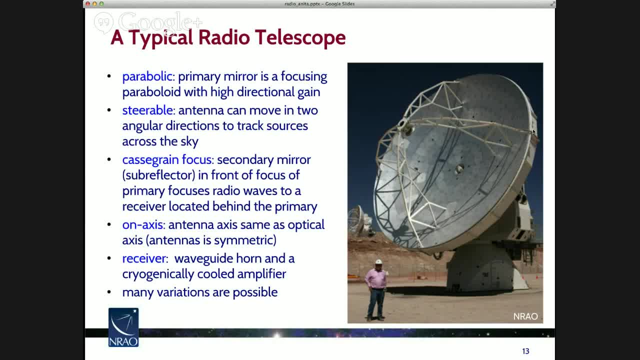 And this is kind of the general scheme of most radio telescopes. but many, many variations are possible, So many variations that I don't even want to start to get into it. but I'll just describe one because it's kind of a fascinating one. 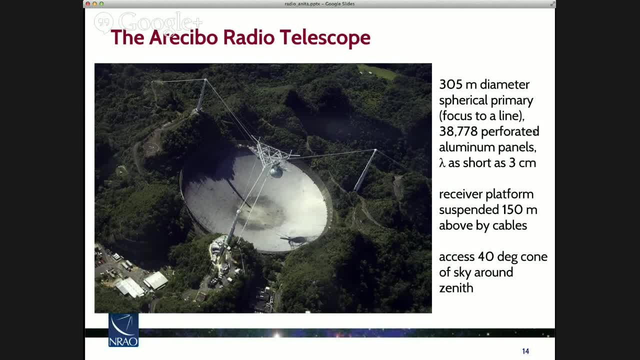 and you may have seen it before, It's currently the largest radio telescope in the world, the Arecibo radio telescope in Puerto Rico. This is a 300-meter diameter spherical primary, so it's not a paraboloid, which means it focuses to a line and not to a point. 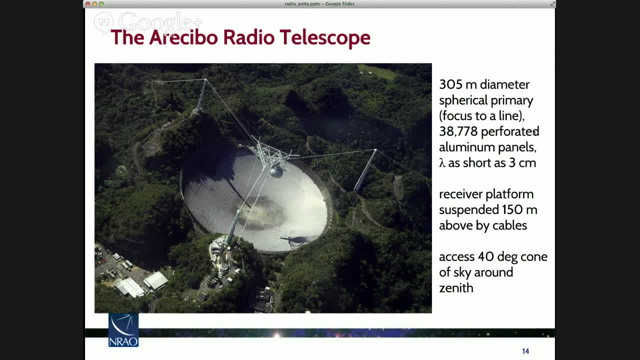 So that's an interesting thing to deal with. at the receptor level, It's made of an incredible number of perforated aluminum panels- more than 38,000 of them- and it can reflect radiation as short as a few centimeters. Now it reflects the radiation up. 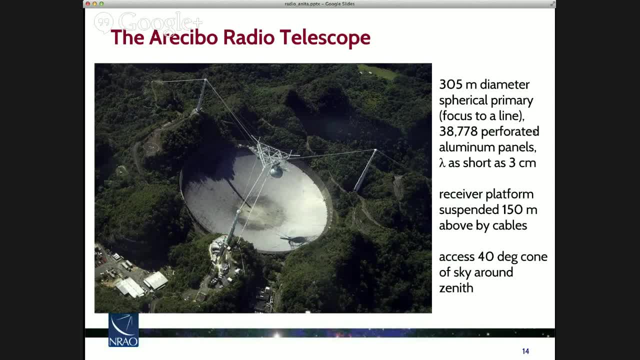 to a receiver platform which is suspended 150 meters above the dish by cables and that can move around to track the source over a 40-degree cone of the sky, around the zenith straight up. So you can see that this has got all the same elements. 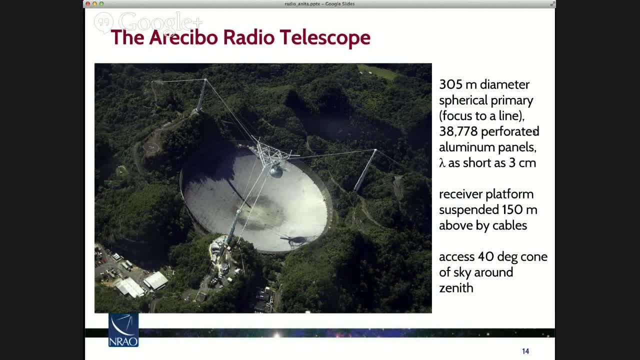 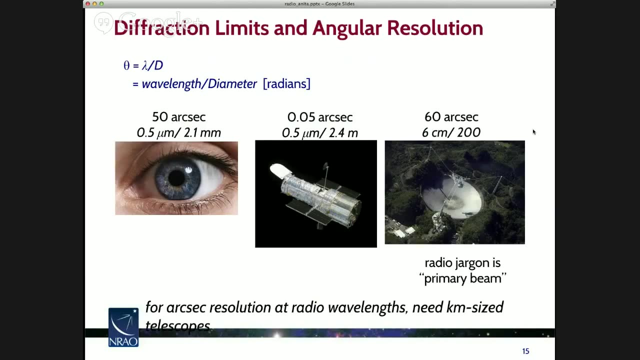 of that abstract radio telescope that I mentioned, but it's a very different sort of implementation and there are many, many other variations which don't even use dishes but use dipoles on the ground and whatnot, that are even completely different. Okay, 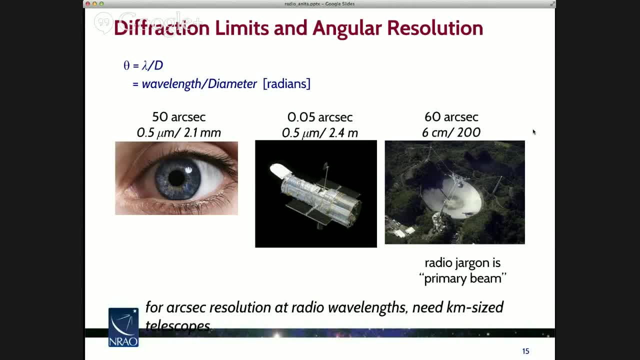 Now, that's a very big telescope but there's a big issue in radio astronomy and that is angular resolution. So I'm sure you're all familiar with Rayleigh's criterion that the diffraction limit of a telescope is given by the number of wavelengths. 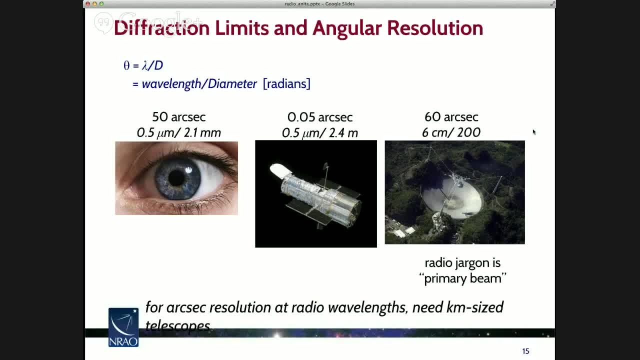 divided by the diameter of the telescope in units of radians. So if you think of your eye as a telescope and you're observing in the optical, let's say half a micron, and the diameter of your pupil is a couple millimeters. 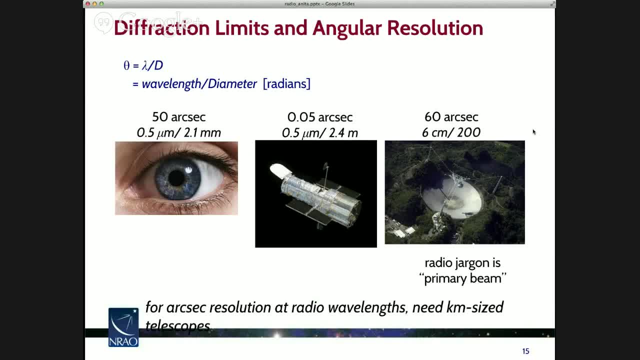 then the resolution of your eye is something like it's about 50 arc seconds, about one arc minute, and if you think about, say, looking at the moon with your eye, you can, you know, start to resolve some small features. 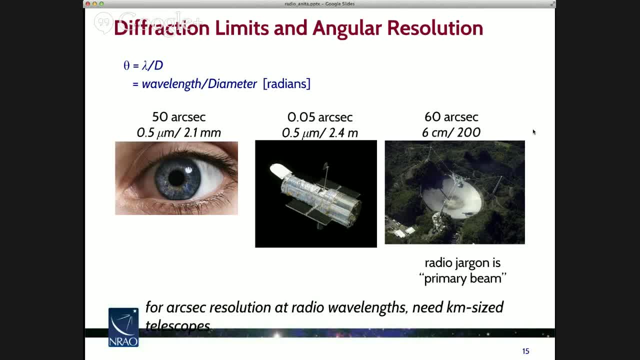 but they're limited. If you think of a really sharp optical telescope like the Hubble Space Telescope, it's observing at the same wavelength as your eye- half a micron- but instead of being two millimeters in diameter, it's two meters in diameter. 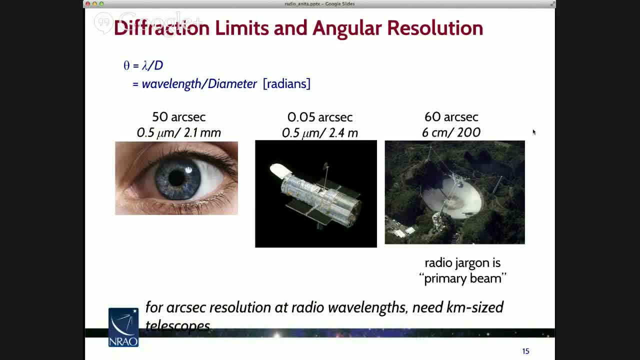 and so it's a hundred times better in resolving power down to 50 milli-arc seconds. so that's really pretty good, and that's great for astronomy, because a lot of things are small. Now, how about the Arecibo radio telescope? 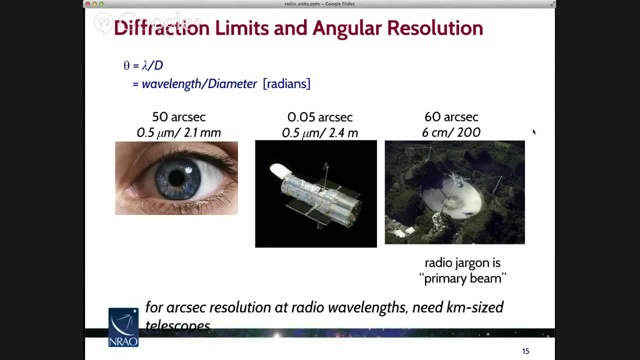 So suppose you're observing at six centimeters and now the effective area that you can use that actually reflects up to the receiver is something like 200 meters. the resolution of that is 60 arc seconds. It's just about the same as your eye. 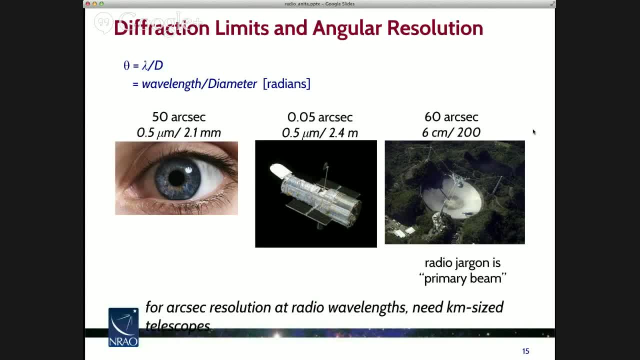 So that's about as big a radio telescope as you can imagine making, and its resolution is no better than your eye. So if you want arc, second or better resolution at radio wavelengths, you need kilometer-sized telescopes, and that was realized early on. 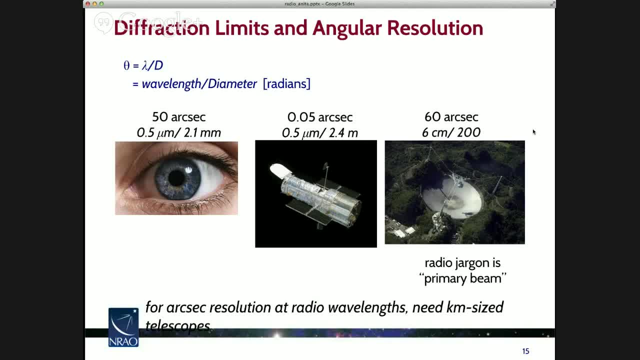 but it's a big challenge because it's hard to make a single telescope that's a kilometer or many kilometer size, and that's why synthesis telescopes came to be. I should mention that the radio jargon for the resolution of a single element. 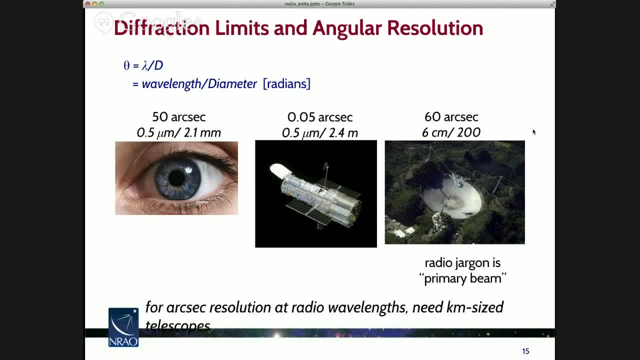 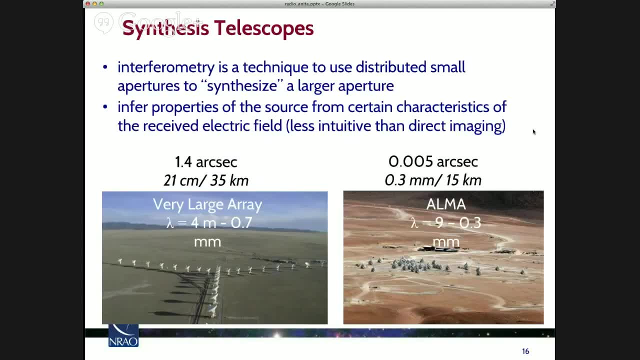 like the Arecibo telescope, is the primary beam. so you'd say the primary beam size is 60 arc seconds for Arecibo. Okay, so synthesis telescopes? Well, interferometry is a technique to use distributed small apertures. 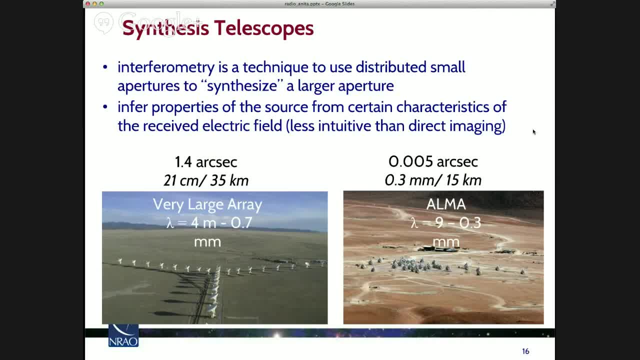 use lots of little telescopes to synthesize a larger telescope, a larger aperture. So I have two examples here on this slide. On the left is the Very Large Array. This is a very famous radio telescope located in New Mexico in the United States. 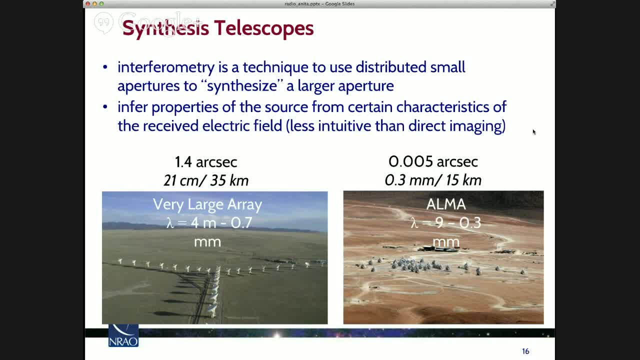 It operates at wavelengths from a few meters down to a little bit less than a centimeter, and it can extend to be 35 kilometers in diameter. So if you imagine you're observing at 21 centimeters, that was the wavelength of the hydrogen spin flip line. 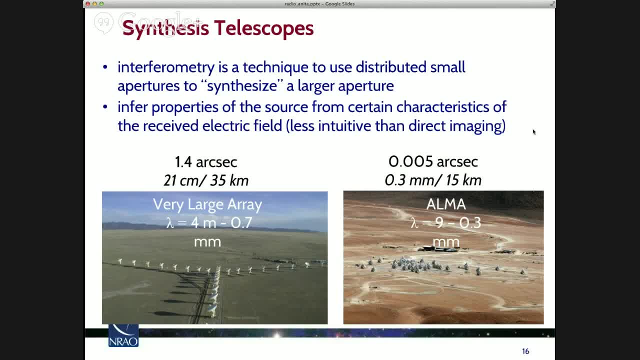 then you could make images with a resolution of 1.4 arc seconds. So now you're getting down to an interesting amount of resolution, but, as you can see, you need a telescope that's 35 kilometers across. That's pretty big. 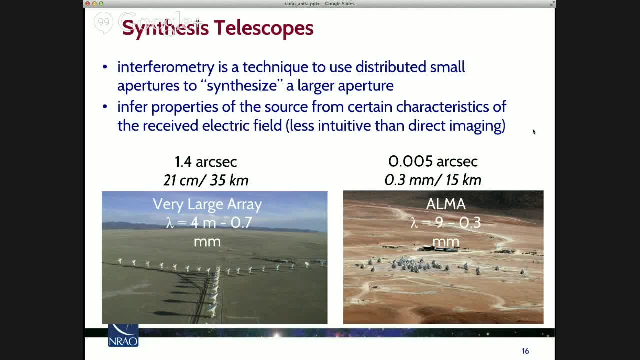 And the newest of these synthesis telescopes, these large synthesis telescopes, is ALMA, which operates in the millimeter and submillimeter part of the spectrum. It has maximum size of 15 kilometers and at the shortest wavelengths that's down to 5 milli arc seconds. 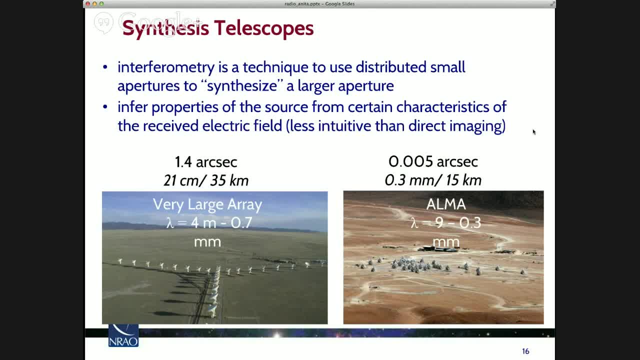 actually an order of magnitude already better than the Hubble Space Telescope, if you're interested in certain kinds of small sources. Now the way synthesis telescopes work is not exactly the same as the way single element telescopes work, because obviously you're not capturing. 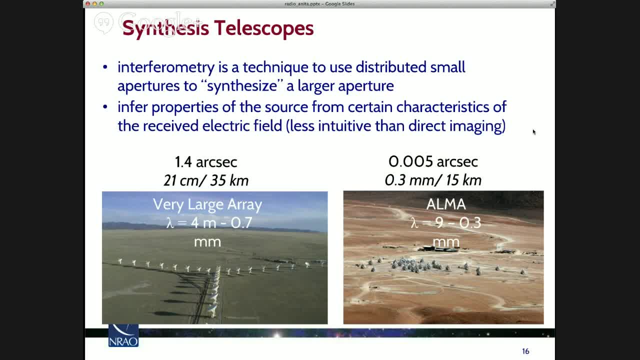 all of the same information when you only have a small fragment of the telescope aperture. So, indeed, what happens here is that you're inferring properties of the source in the sky from certain characteristics of the received electric field that are not just the intensity. 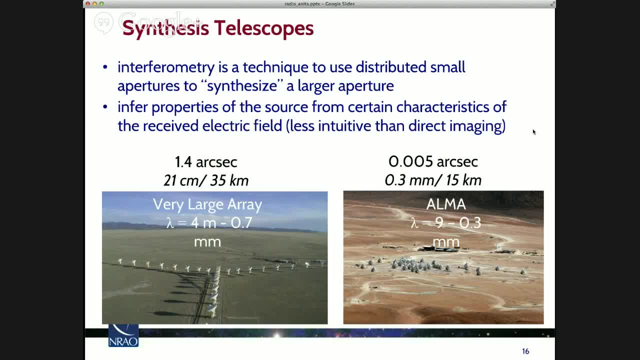 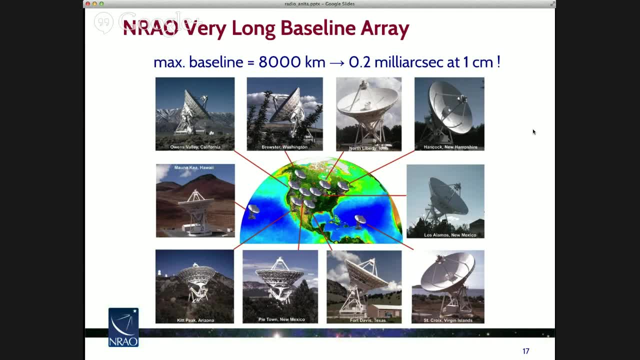 So this is quite a bit less intuitive than direct imaging, but I want to give you a feel for that. Oh, I have one more example. first, The Very Long Baseline Array. this is a fascinating telescope, So it has a maximum size. 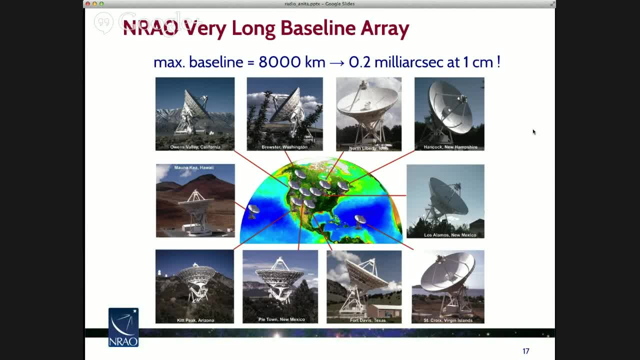 of the size of the Earth, 8,000 kilometers, And so if you're observing at a wavelength of one centimeter now, the resolution is already 0.2 milli arc seconds, which is quite incredible. Now for this to work, you can imagine. 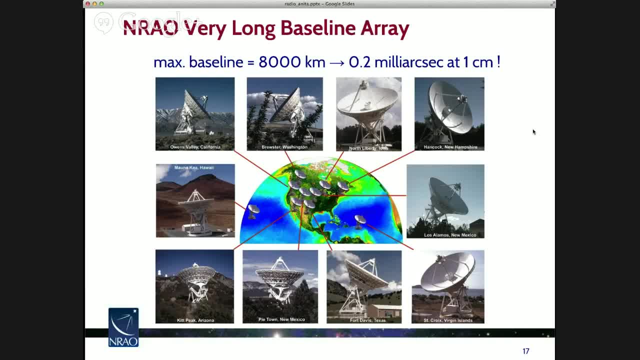 you can't actually physically connect all of these telescopes, but you can record the information at each telescope and then combine it later to achieve this resolution and infer certain properties of the sources. All right, So now we're going to transition and talk in more detail. 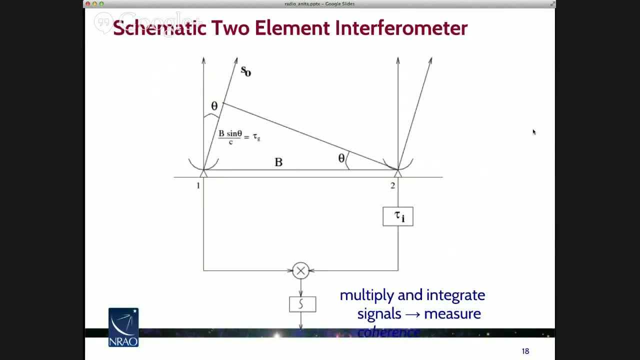 about interferometry. Here's our schematic two-element interferometer, So you can imagine each one of these telescopes. one and two are abstract radio telescopes that do some sort of collection of the radio waves and detect them. So these telescopes- 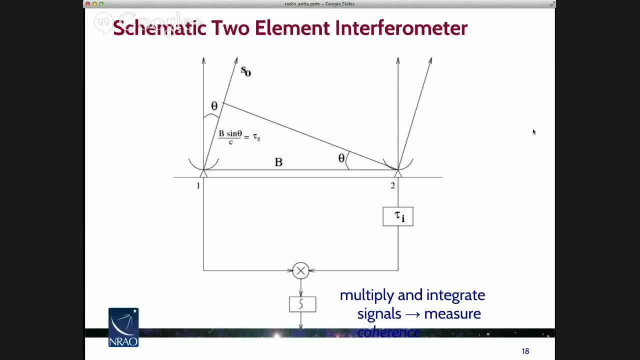 are pointing at a source, at a direction which is labeled by the specter S0, which is at an angle theta from the zenith, And the way that the two-element interferometer works is that the telescope on the left you can see the signal gets there. 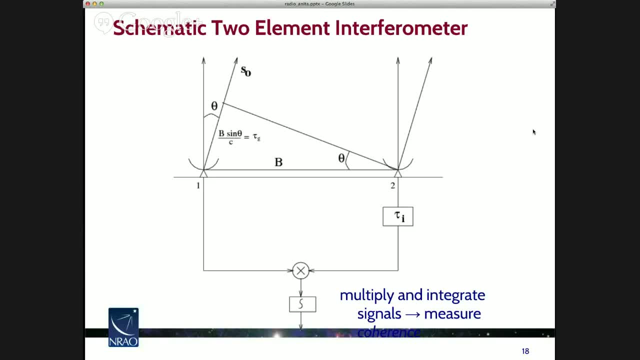 a little bit later than the telescope at the right. There's a time delay which is labeled on the figure as B, sine theta over C, And so what one does is one delays the signal from telescope two. in this case, that's the tau that's listed there. 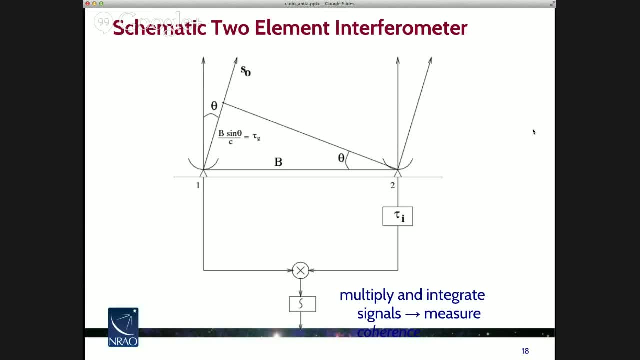 and you multiply the signals and integrate them, And what you measure- and I'm sorry that my font was converted here- is something called coherence of the signals. So what the interferometer measures is not intensity directly, but coherence. We haven't really had too many equations. 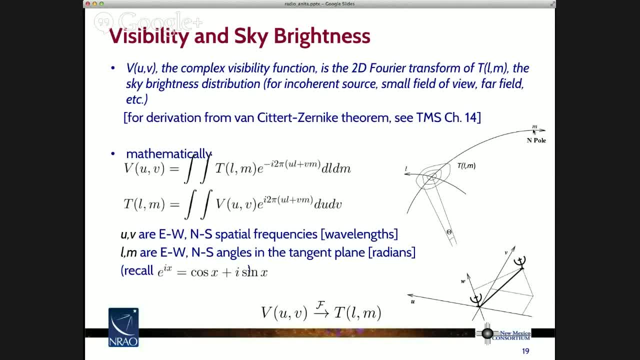 in this talk. Here's the one slide that has a very important equation. So what is this coherence? I want to give you some feel for that. There's something that radio astronomers call the visibility. It's a complex visibility function, And what this is? 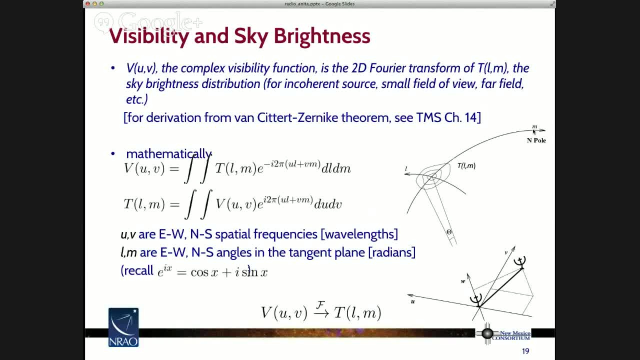 effectively is the two-dimensional Fourier transform of what the emission is on the sky And if you want a derivation of where this comes from for the two-element interferometer, one can look at that reference I mentioned with Thomson, Moran and Swenson. 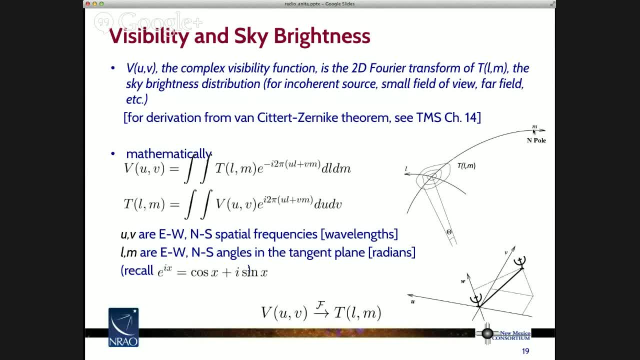 in Chapter 14.. There are a few different ways one can derive this. I think this is one of the more transparent ones, but it still takes several pages of equations, and so I'm not going to go into that. for this talk, There are limitations. 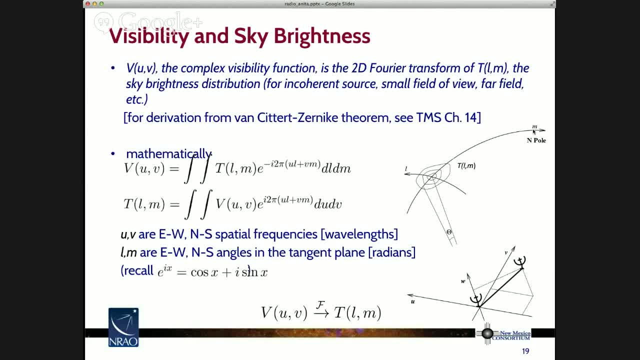 as to when this applies and when it doesn't. But if you look at the figure on the right, this describes the basic geometry and I can explain the equation that comes on the left. mathematically, Our two-element interferometer there is on the ground. 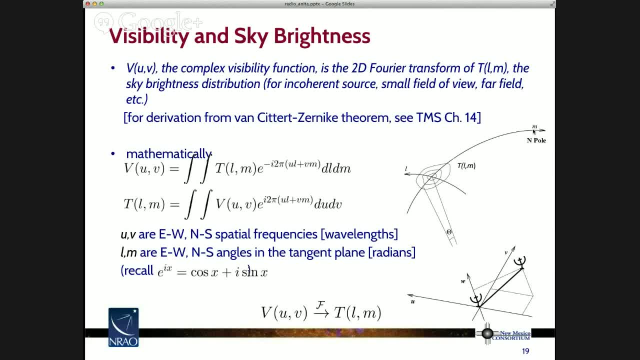 and there are two coordinates, u and v. u points east and v points north, And you measure the separation of these telescopes on the ground in terms of number of wavelengths in u and v. So they're the east, west and north. 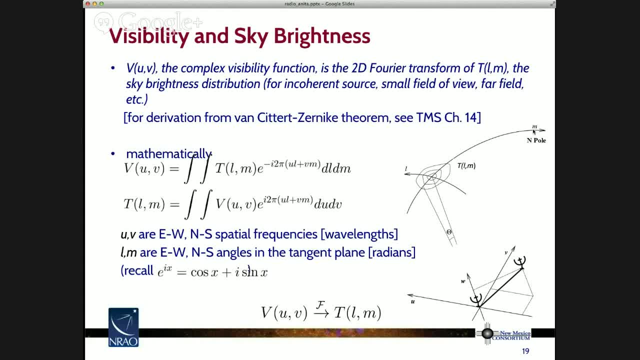 south spatial frequencies, they're called- measured in wavelengths on the ground. Then if you go to the sky plane, you can see that there's a double integration, which is called tlm, on this figure. Now, l and m are angles on the sky. 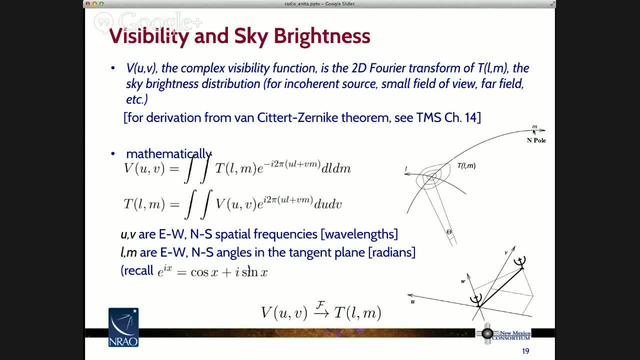 and so they're the east, west and north, south angles in the plane that's tangent to the curved sky. Now, what is this visibility? So this visibility as a function of u and v on the ground, is this double integral? 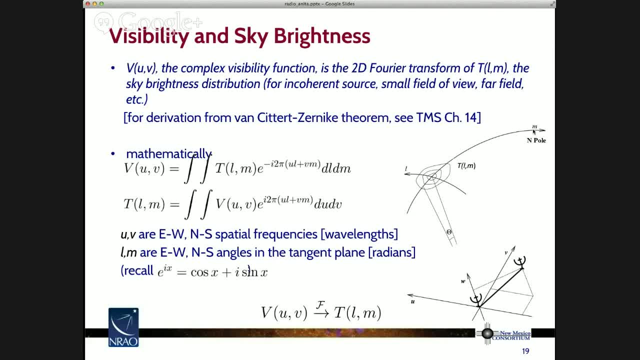 of tlm on the sky times, this exponential factor, u l plus v, m, then integrated over these angles. So, if you remember, this e to the 2 pi i times these other factors is just a series of sines and cosines. 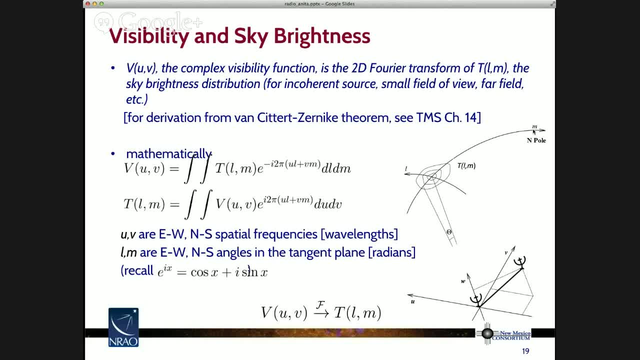 e to the i x is cos x plus i sine x. I'm sure you remember that. So this visibility is the sky brightness multiplied by a bunch of sines and cosines and then integrated, And what that actually is in detail is a two-dimensional Fourier transform. 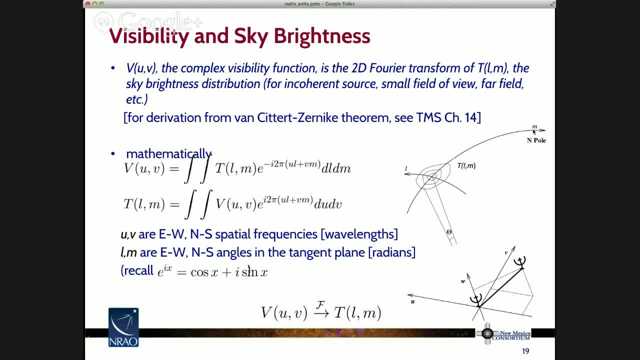 So at the bottom of the slide I have a shorthand notation for this equation. that v u v is this Fourier transform, that little arrow with the f of tlm, And one of the properties of the Fourier transform that I'll describe in a moment. 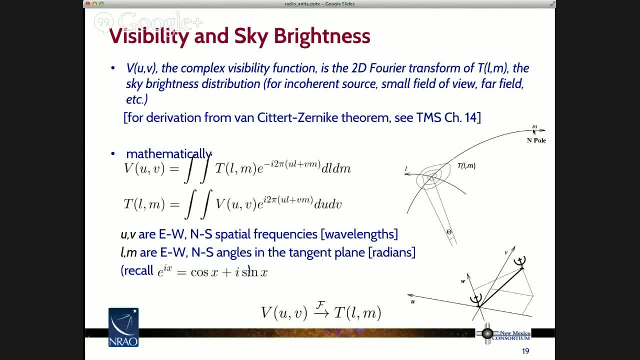 is that it also works the other way. The sky brightness distribution is the Fourier transform of the visibilities. So this interferometer is measuring coherence, It's measuring the visibility function. So for a particular separation of antennas at a point u and v, 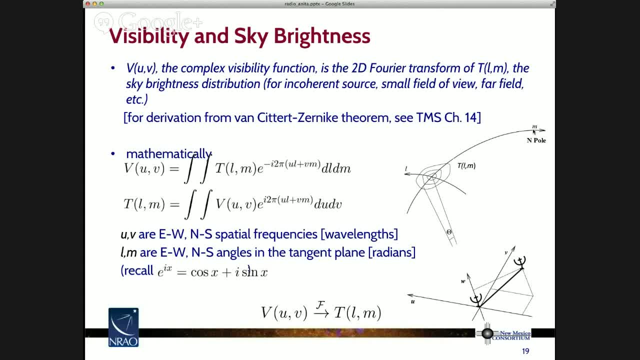 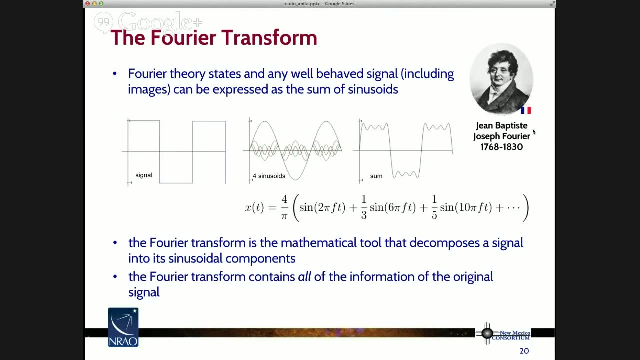 one gets some measure of the Fourier transform of the sky brightness, tlm Alright. So you can see Fourier transforms are important. So I want to spend a few minutes discussing in more detail the Fourier transform. So I'm sure some of you know everything about Fourier transforms. 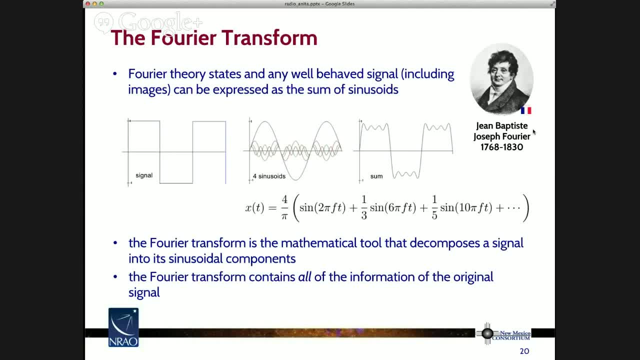 Some of you may know nothing, So hopefully, for those that know something, this will be a good review. So basically, Fourier theory states that any well-behaved signal, that includes images, can be expressed as the sum of sinusoids. And here's a picture of our hero. 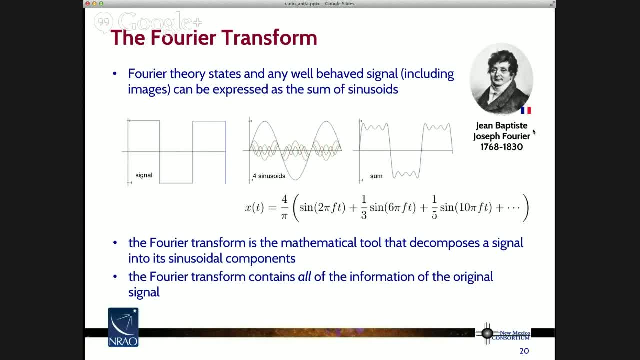 Jean-Baptiste Joseph Fourier, a Frenchman from the 18th century. So if you imagine a signal like a square wave, you can represent a square wave kind of by four sinusoids. If you sum them up appropriately, you get something that kind of looks like a square wave. 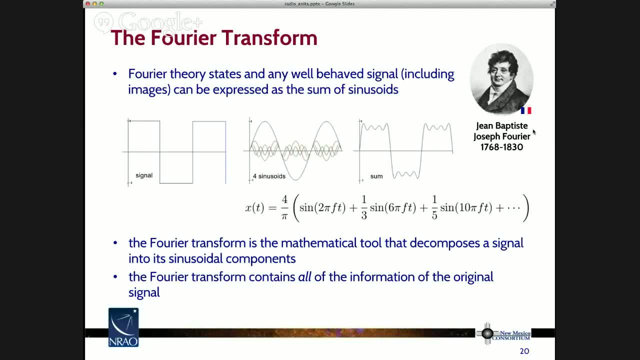 And in fact you may know from your Fourier analysis classes that you can approximate the square wave by an infinite number of sine waves. It's just that to get those sharp edges you need a lot of little tiny waves, so you need a lot of terms. 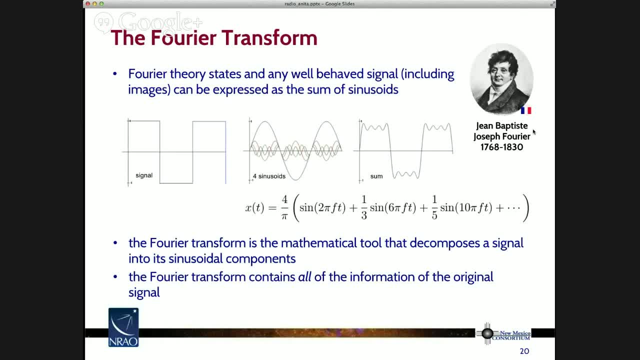 in your function. But the Fourier transform at its heart is just a mathematical tool that decomposes a signal, any signal, into a sinusoidal component, And what's important to remember is that the Fourier transform of a function, of a signal, contains all of the information. 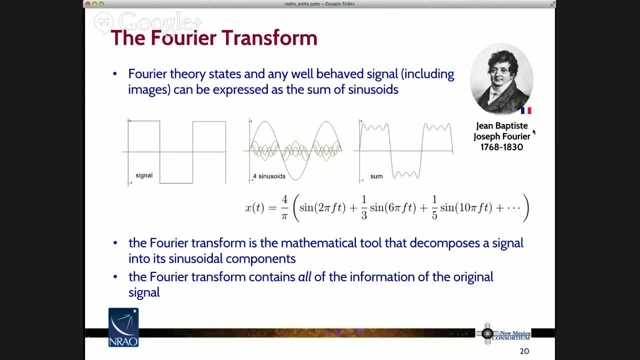 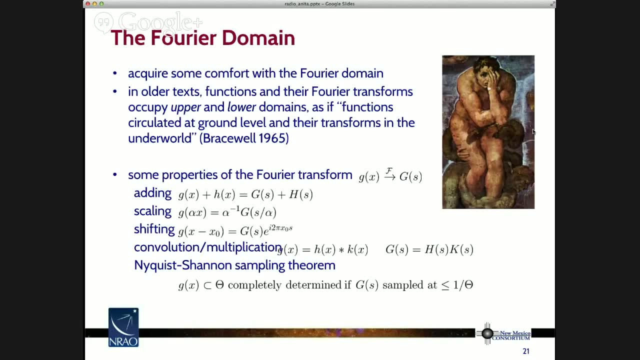 of the original signal. So if you know the Fourier transform, then you actually know the original Okay. So if you want to do radio astronomy and in particular interferometry, you really want to acquire some comfort with the Fourier domain. If you look at 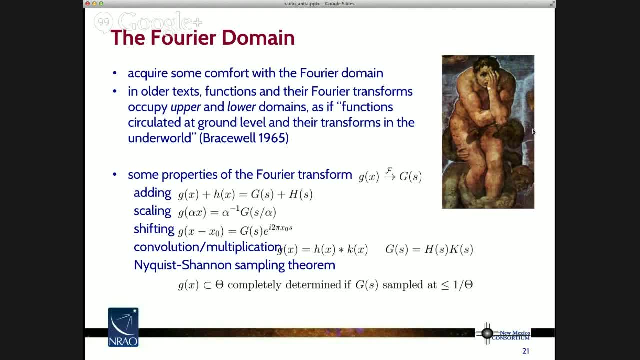 old textbooks, functions in their Fourier transforms are said to occupy upper and lower domains, as if- and this quote is from Bracewell, one of my favorites- functions circulated at ground level and their transforms in the underworld, And you can decide whether it's the visibility. 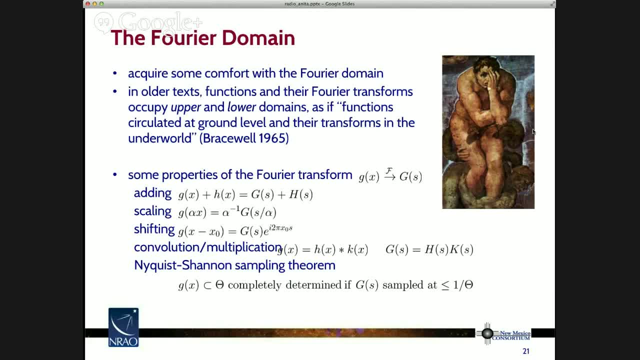 or the sky brightness that's in the underworld at the end of the lecture. So some properties of the Fourier transform are that it's linear. So I've written here: the small g is the Fourier transform of the large g. so if you have two functions, 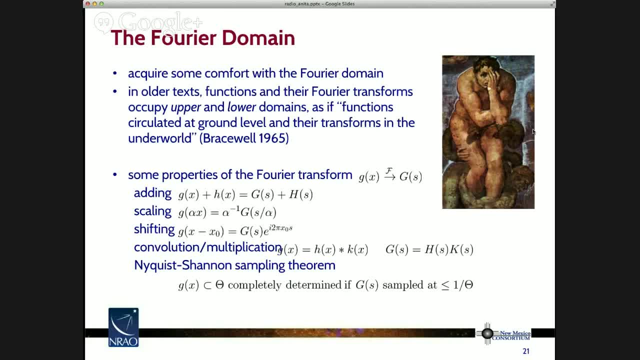 say g and h, if you add those two functions together and get a new function, the Fourier transform is just the addition of the Fourier transform of the individual functions, So they simply add. so that's useful. There's also a scaling property if you multiply. 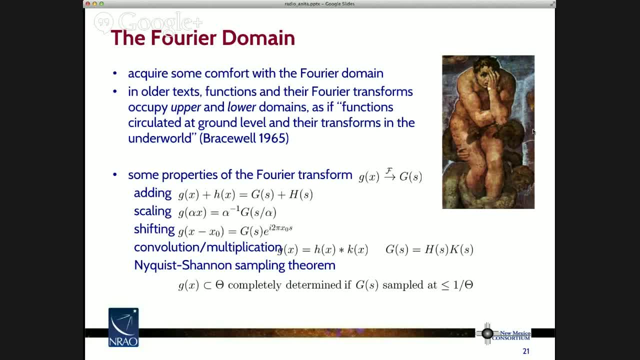 the coordinate by some value, alpha. here you scale it, then the Fourier transform is also scaled, but by the inverse of that alpha There's a shift theorem. If you shift the coordinate, then you just add a phase term to the Fourier transform. 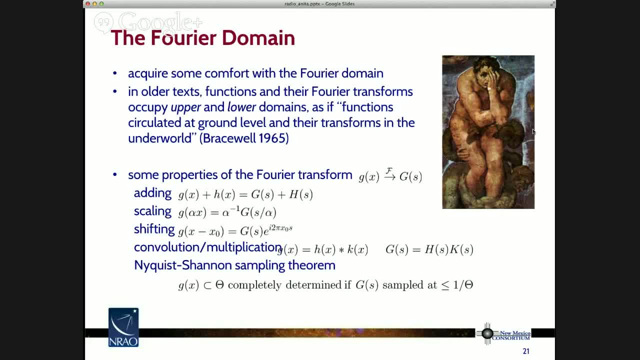 You just change the phase of the sinusoids And there's a convolution multiplication theorem, that is, if a function is the convolution of two functions, then its Fourier transform is the product of the Fourier transforms of those functions. And finally, in one version of the sampling, 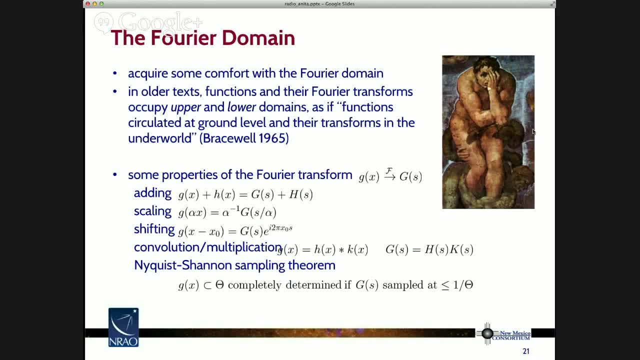 theorem. if you have a function that's restricted to a domain, say theta, it's completely determined if the Fourier transform is sampled at intervals of one over theta. So you don't need to sample every part of it, you just need to satisfy. 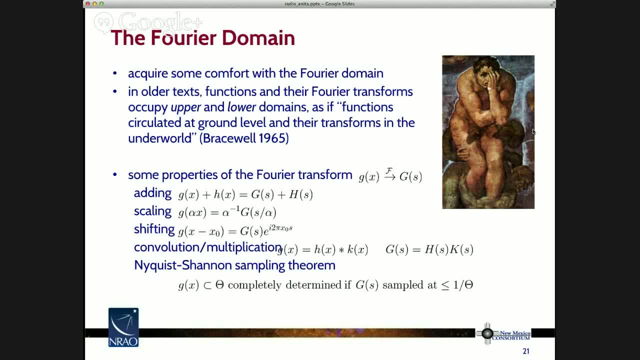 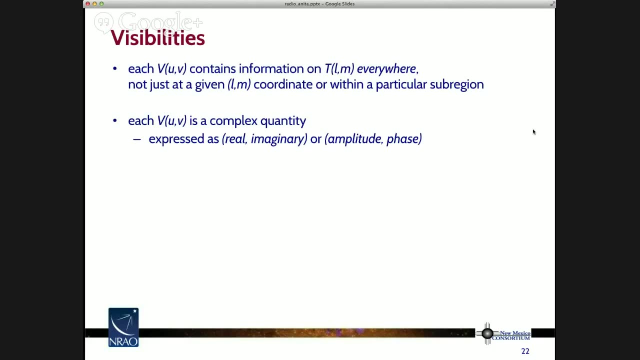 the sampling theorem to completely determine the function. So those are all mathematical properties of the Fourier transform that are useful to keep in mind, And in some examples that are coming up you'll see how these come into play. Okay, Another word about visibilities. 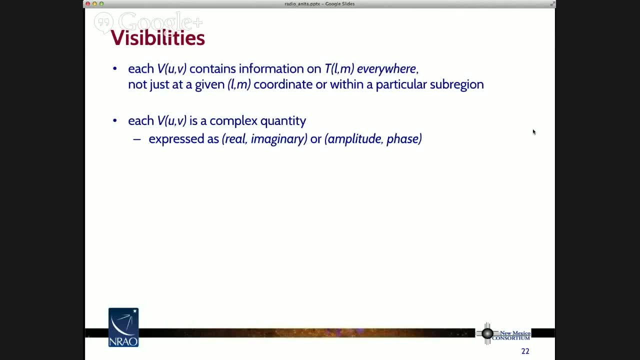 As I mentioned, each visibility- so at some UV point- contains information on the sky brightness everywhere Right. Because of the sinusoidal nature of the phase term, you can see each point in the UV plane, as it's called, in the visibility domain. 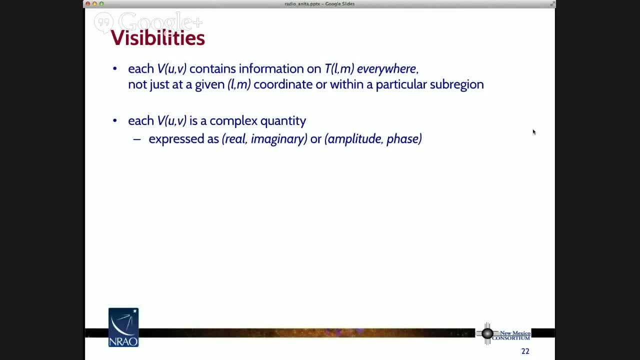 has information on the sky brightness everywhere in that domain, Not just at one place in the sky brightness distribution or within a particular region, but everywhere. The other thing is that you remember the eye. each visibility is a complex quantity, So it's often expressed. 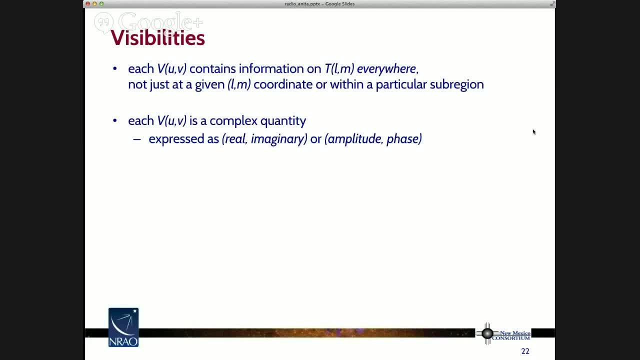 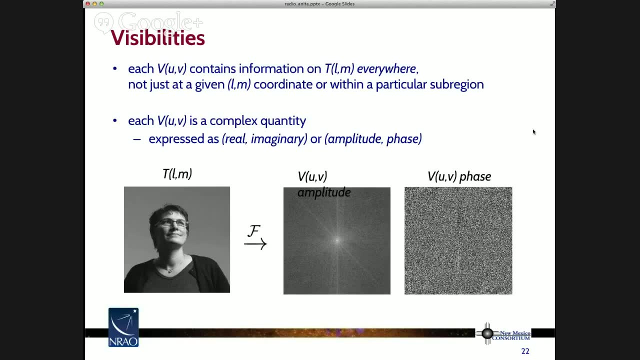 as a real and imaginary part, as a real part and an imaginary part or as an amplitude in that phase. Either one works. So here's an example of a Fourier transform of an image. We have here an astronomer represented as sky brightness. 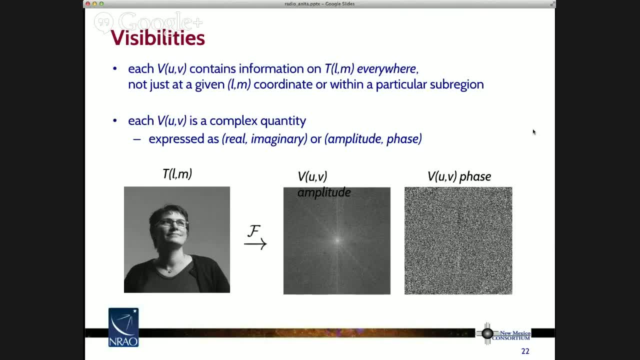 T of lm. If you Fourier transform that image, you get information, visibility at a whole bunch of UV points. you have amplitude and you have phase. So you see, that's one way to do it, Or it could be real and imaginary. 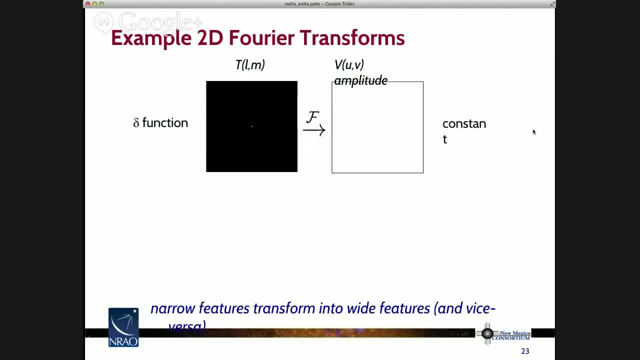 So I'm going to go through a few examples of Fourier transforms to give you a little more intuition about them. A delta function is kind of the narrowest function you can have. So if you imagine sky brightness, that's really peaky a delta function. 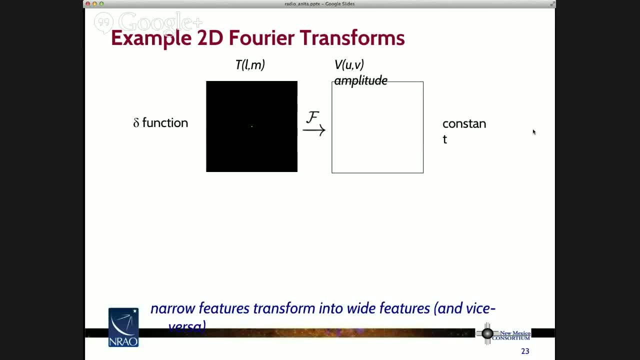 if you Fourier transform it, it's a constant. It has the same visibility amplitude everywhere. A Gaussian transforms into a Gaussian And a narrow Gaussian transforms into a wide Gaussian. So narrow features transform into wide features and vice versa. So if you see something that's narrow, 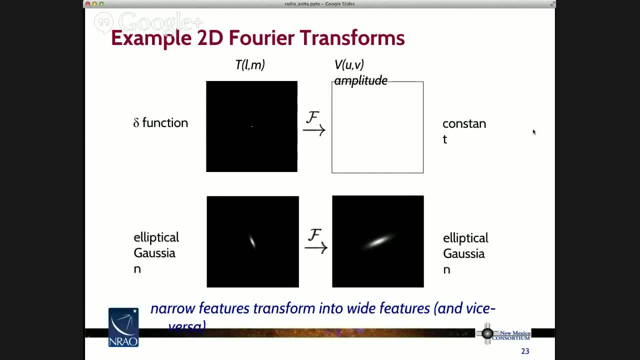 in one domain, it's going to be broad in the other domain. So here's an elliptical Gaussian. You can see it's narrow in one dimension and broad in the other. And if you look at its Fourier transform, it's going to be broad in one dimension. 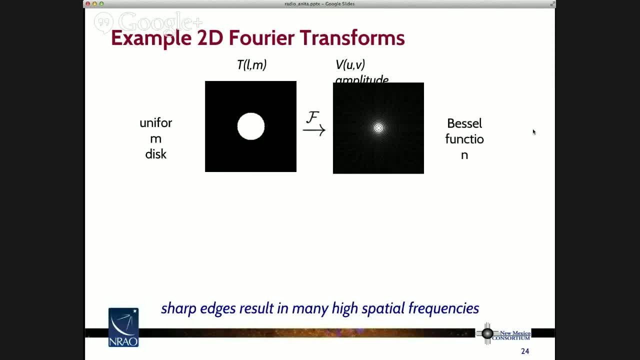 and narrow in the other. Okay, Here's a uniform disk. When you Fourier transform that, you get a Bessel function. So hopefully you can see the series of rings that come around from the Bessel function. And what does this mean? 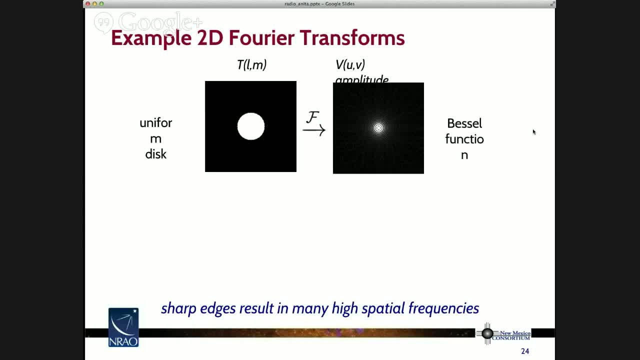 The disk has a sharp edge, And so if you want to represent that sharp edge, it means you need a lot of high spatial frequencies And the Fourier transform out at large u and v in order to represent that sharp edge. So this is analogous to that square wave. 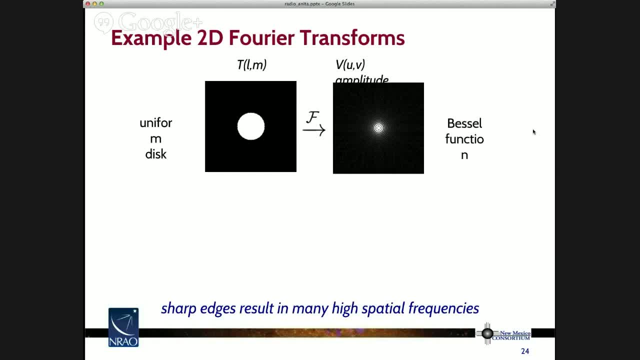 that I showed you earlier. If you really want to get the sharp edge, then you need all of the visibility plane. Here's another example You might think about. what's the Fourier transform of this look like? Think about that for a minute. 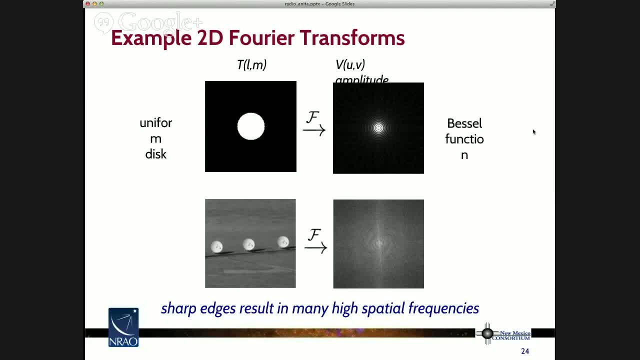 Here's the answer. It looks a lot like the Bessel function above. So why is that? That's because the spatial frequencies you need to make three disks are pretty much the same as the spatial frequencies you need to make one, And it's the phase. 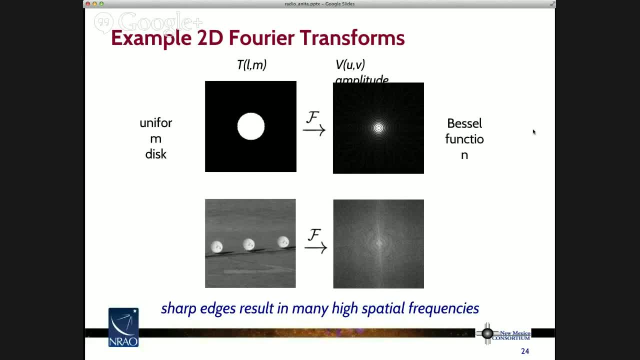 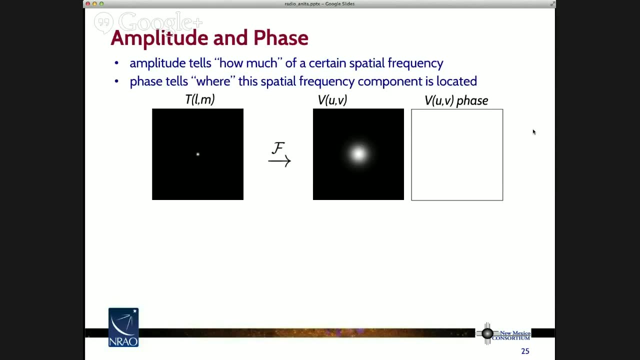 information that I'm not showing here, that's telling you where that stuff is located. So this is, I think, perhaps the biggest trap in Fourier transforms and radio interferometry: It's understanding the nature of amplitude and phase, And so I'll try to give you a little. 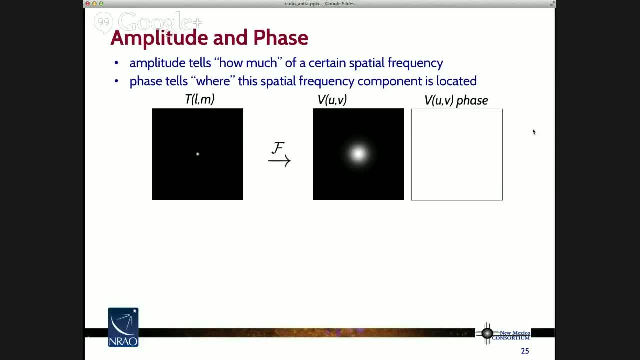 bit of an example here. Amplitude tells you how much of a certain spatial frequency you need. So here's our little Gaussian On the left. Fourier transforms into a big Gaussian and the phase is constant. Why is the phase constant? It's telling you where these spatial frequencies. 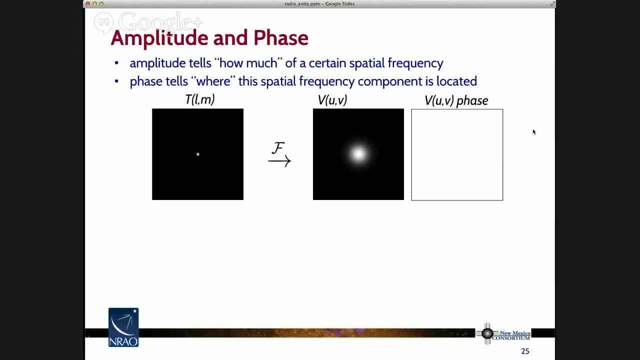 are located. Our little Gaussian is in the center of this image, And so the phase information is kind of not very interesting. If I shift the source over a little bit away from the center, then the amplitude of the visibility are exactly the same. 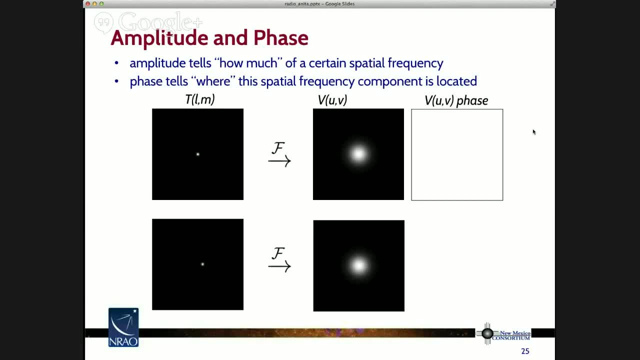 right, You need the same sine waves to make the small Gaussian, whether it's shifted or not, But the phase is different. Oh great, And unfortunately the slide isn't showing that, But you can imagine that the phase is different. 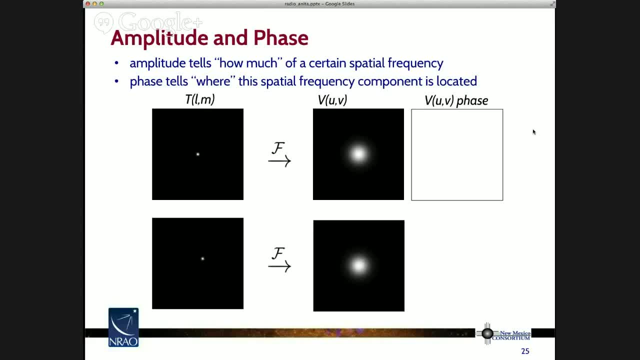 And if I were to move the source in a different direction and do the Fourier transforms again, the amplitudes are the same and the phase that you can't see is different. Okay, We'll have to fix that, All right. So let's review a little bit. 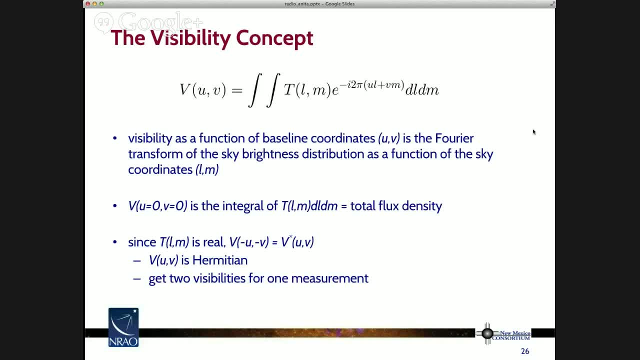 this concept of visibilities. This is the one equation. remember The visibility as a function of u and v. so those are spatial frequencies on the ground measured in wavelengths. is this double integral over sine waves of the sky? brightness distribution where L and M are angles on the sky. 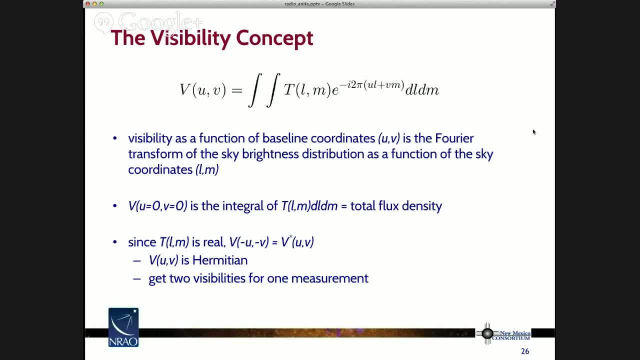 So there are a few things to notice. One is, if you put zero in for u and v- right, so you're at the origin of the UV plane, then what you get is just the integral of the sky, brightness distribution And in radio astronomy. 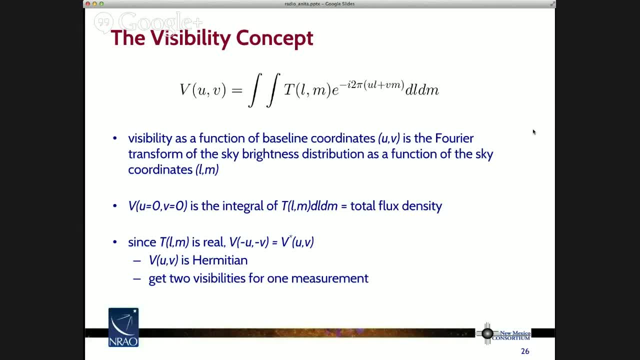 that's just the total flux density. So the visibility right at the center of the UV plane is just the total flux density. Another thing to notice is that because sky brightness is real right, it's not imaginary. if you put in minus u and minus v. 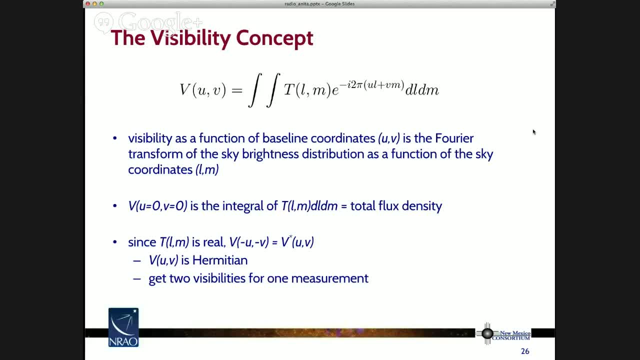 then you get the conjugate version of Vuv, So v. the visibility is said to be mathematically Hermitian and that means you get two visibilities for one measurement, That is, if you make a measurement at u and v. 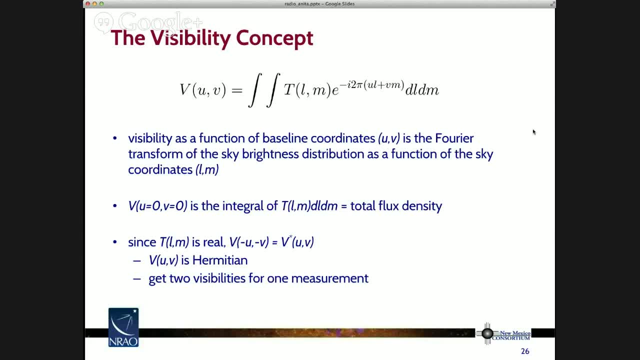 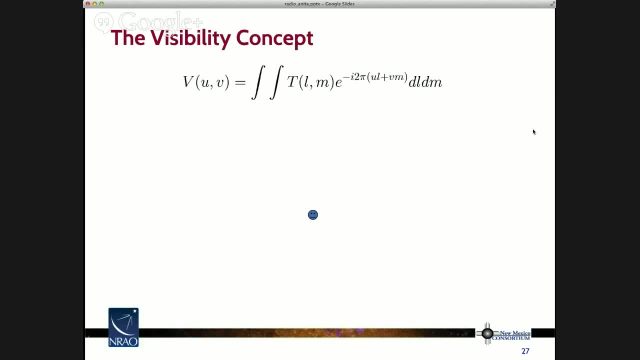 you also get the answer at minus u, minus v, So that's convenient for radio astronomy, All right. So this little illustration is to kind of show you what this equation means. So I've said it in words a number of times. I'll say it again. 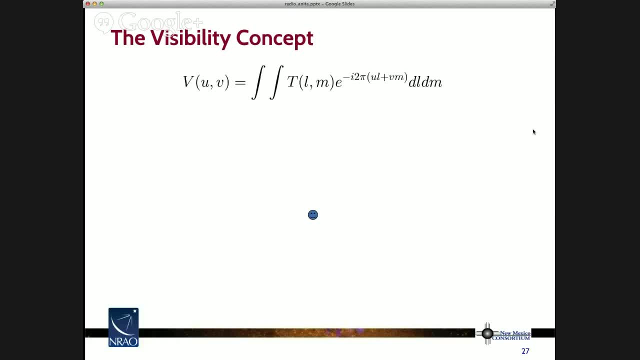 The visibility is the sky brightness multiplied by a bunch of sine waves and then integrated. So this little smiley face here is going to be our sky brightness distribution, our T of lm. Now, if we have an interferometer, then it effectively puts a sine wave on the sky. 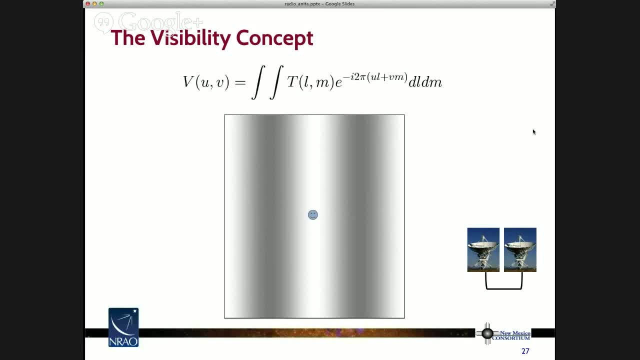 a fringe pattern, as it's called, And it multiplies the sky brightness distribution by this fringe pattern. So you can see the pattern of light and dark is plus and minus of the sine wave. And so you do this multiplication and you get a number. 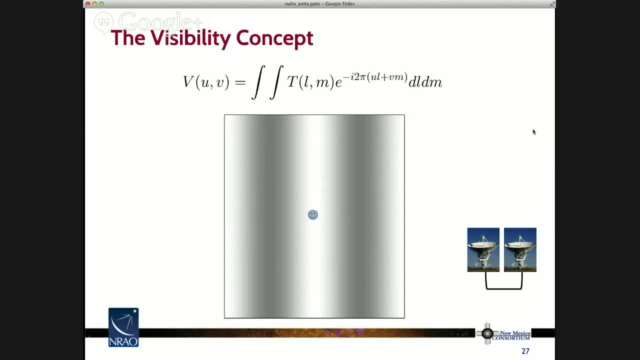 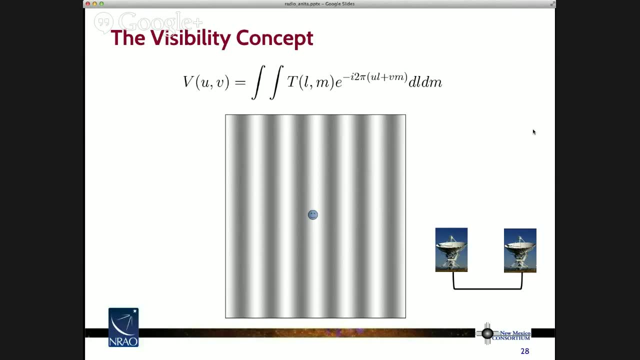 And that's the visibility. So that's all there is to it. If we separate our antennas a little farther on the ground, then we get a different set of sine waves. we get a higher spatial frequency because in this case we've made U bigger. 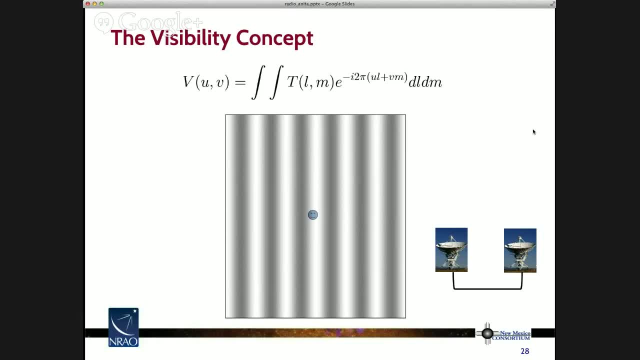 so we have a faster sine wave, And you can see, if you multiply this sine wave by the little smiley face, you get a number, And in fact that number is essentially the same as the number from the previous set of antennas. And then, if we 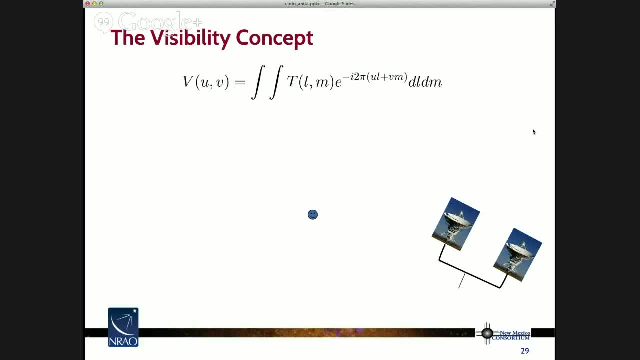 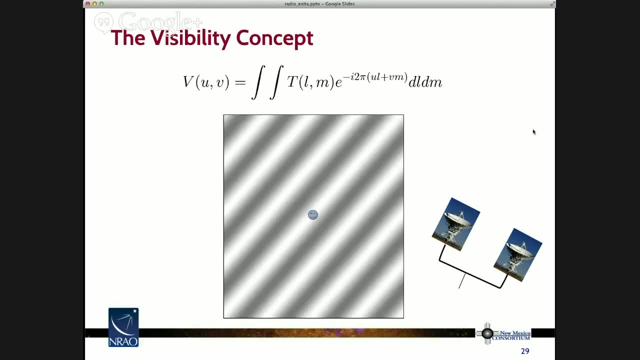 do it again. this time we turn the antennas a little bit, we get the same angle now. Now the fringe pattern is rotated And if we do the same multiplication of the sky brightness by the sine wave, we get a number. Again, it's almost the same number. 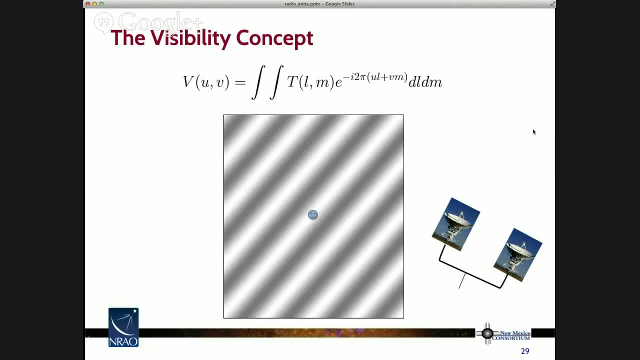 if not exactly the same number. So what is that telling you? That means any separation of the antennas is giving you the same visibility. That's telling you that the source is small. right That it's a point source. Remember the Fourier transform. 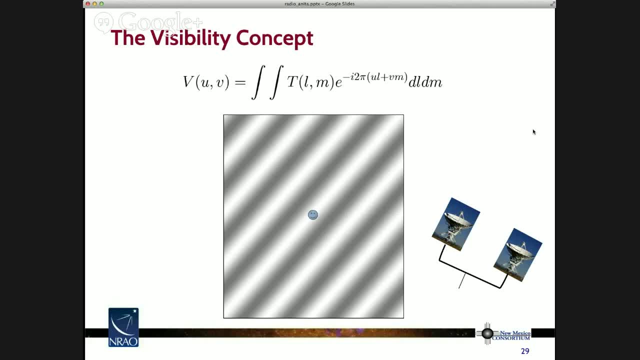 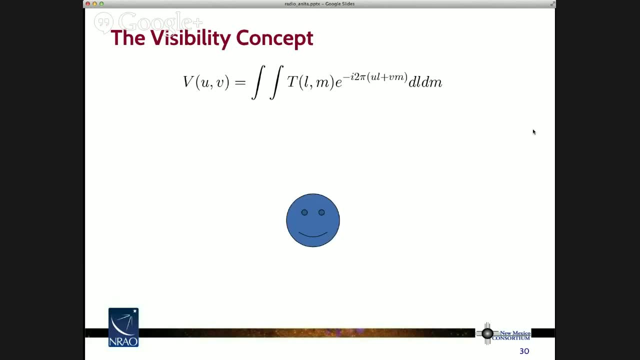 is telling you that there's not much information. besides that the source is smaller than the resolution of your antenna baselines. So, by contrast, here's a bigger source, another happy source, a bigger one If we start with the antennas close together. 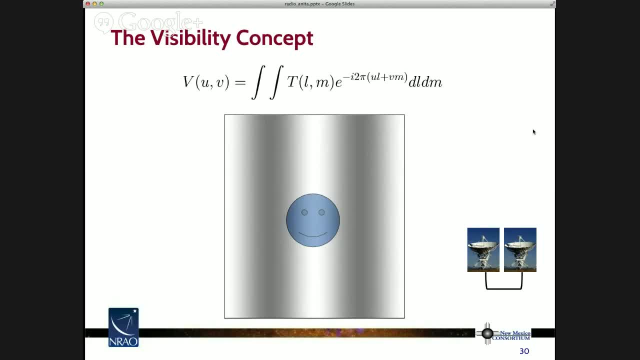 we get the broad sine wave. If we do this multiplication, you can see we get a number. but you can see part of the source is on the right side of the wave and part of it's on the positive part and part of it's on the negative part. 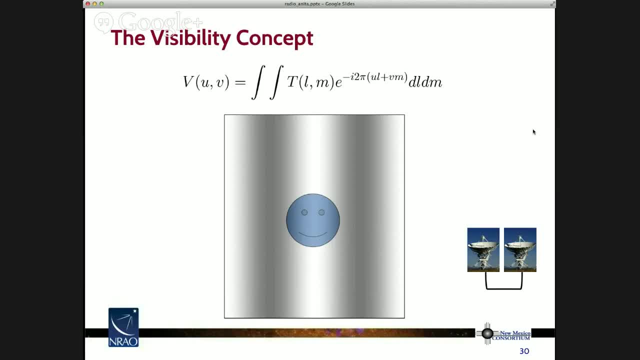 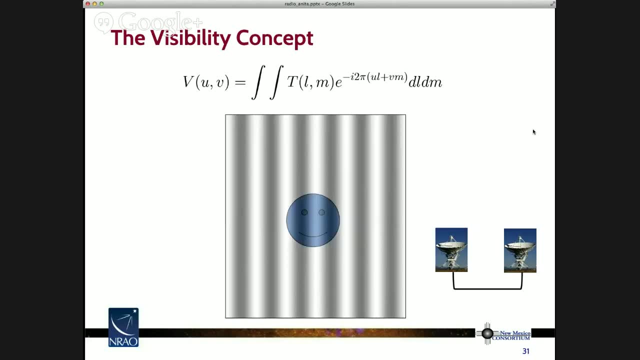 So if we do this multiplication and integrate, then we get a number which is smaller than the total flux. That's to say, the source is resolved. If we move the antennas farther apart and we do the same exercise, now we have a bunch of sine waves. 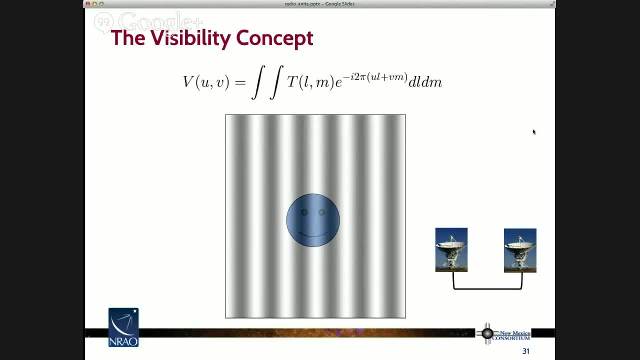 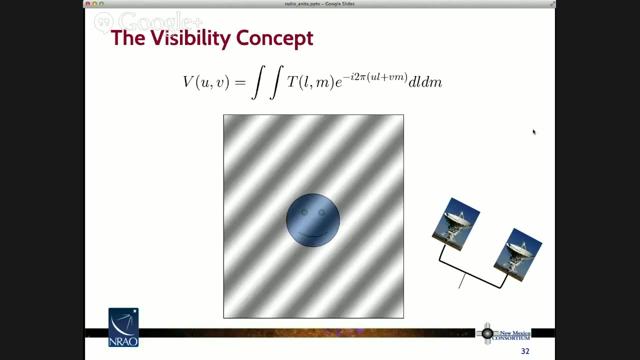 across the source. So we do the multiplication and we get a number that's now probably pretty small, except for the little variations of the eyes and the smile. And if we turn to a different baseline and we do this exercise again, we're going to get a different number. 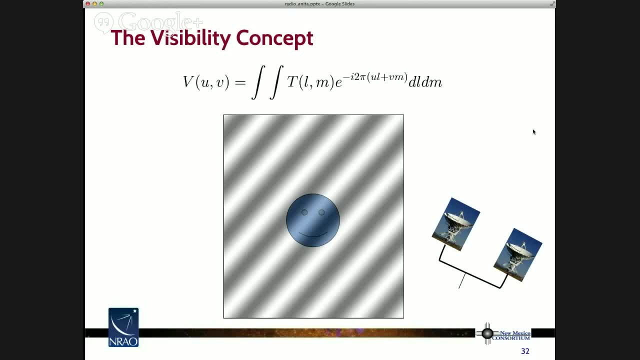 and a lot of the difference in this case is going to be due to the fact that there's this small scale structure on the source, the eyes and the mouth, And so that's the name of the game here- is that, if you can make enough, 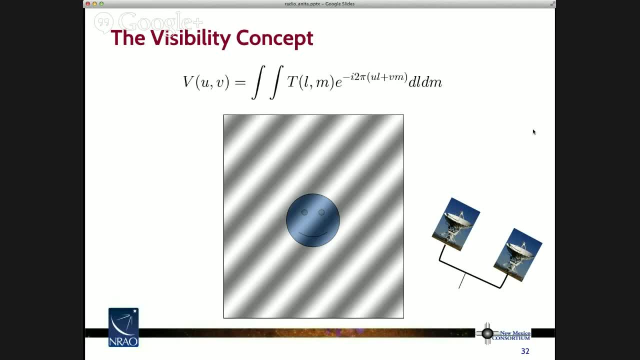 different measurements of the visibility, then you can learn about the structure of the sky brightness. If you made enough different antenna pair measurements, then you could reconstruct the information that you have a smiley face on the sky. So that's aperture synthesis right. 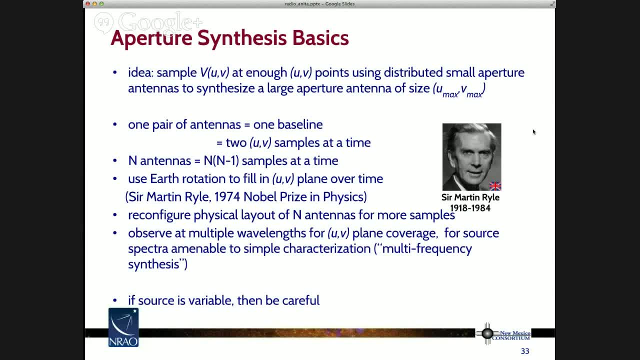 The basic idea is to sample the visibility function at enough UV points using these distributed small aperture antennas to synthesize the resolution of a large aperture which goes out to the maximum UNV that you can measure. So one pair of antennas, one baseline, gives you two samples. 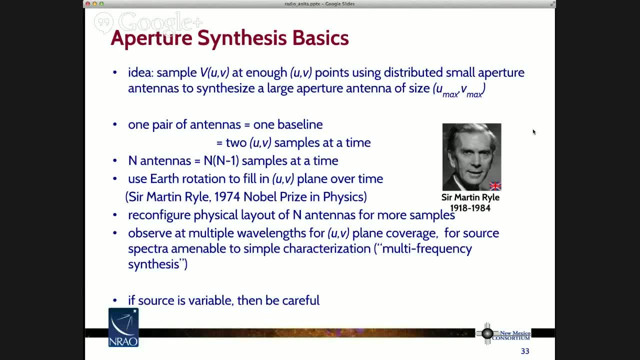 because the visibility is permission at a time. So two samples is not very many if you want to build up all that information. if you had to do it one pair of antennas at a time it would be pretty painful. So if you have any antennas, 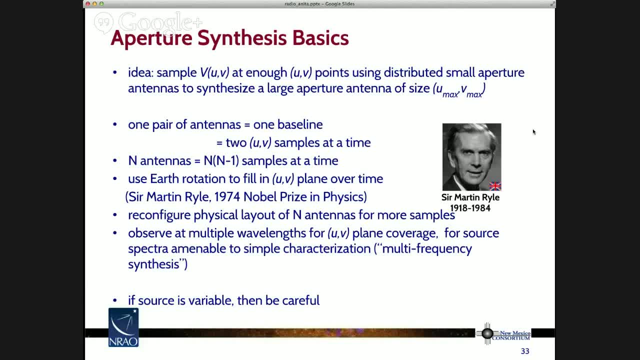 well then, you have n times n-1 pairs, so you get n times n-1 samples at a time. And if you're really clever, you know that the Earth is turning, whether you want it to or not, And so your UNV on the ground. 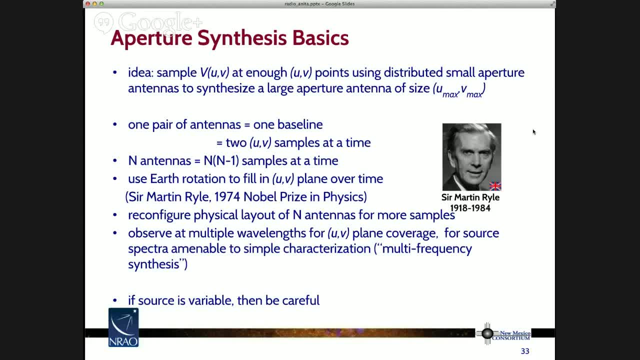 are changing, whether you want them or not, for fixed antennas, And so Earth rotation actually tends to fill in the UV plane, no matter what you do, And, in fact, the realization that one could take advantage of this and make aperture synthesis measurements using a number of antennas. 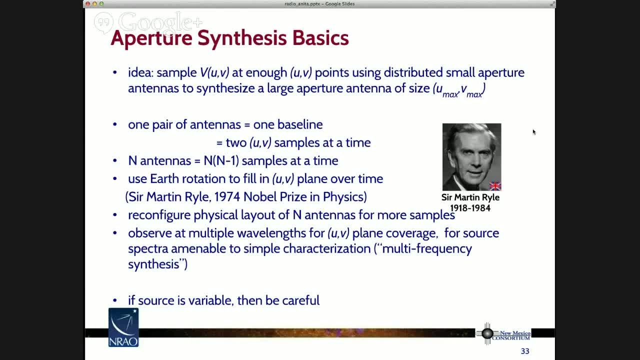 and Earth rotation was a big part of the 1974 Nobel Prize in Physics. Sir Martin Ryle, British, had to balance the French from earlier 1974. So if you only have any antennas then you probably have to move them around to get more samples, that is. 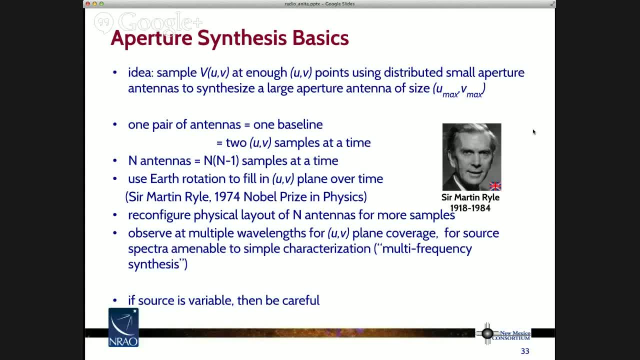 you can reconfigure their physical layout. And another thing you can do: if your source emission is the same at a bunch of wavelengths- which maybe it is, maybe it isn't, you'd have to know- you can observe at multiple wavelengths at once because, remember- 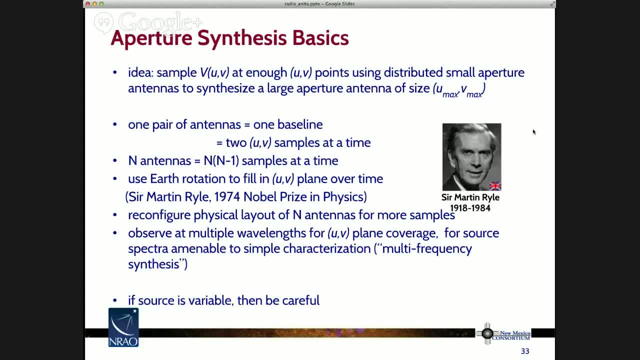 UNV are measured in wavelengths, so if you were observing at multiple wavelengths, you can cover different parts of the UV plane at the same time, and so this is called multi-frequency synthesis. but it only works if you understand the source spectrum and you can characterize it. 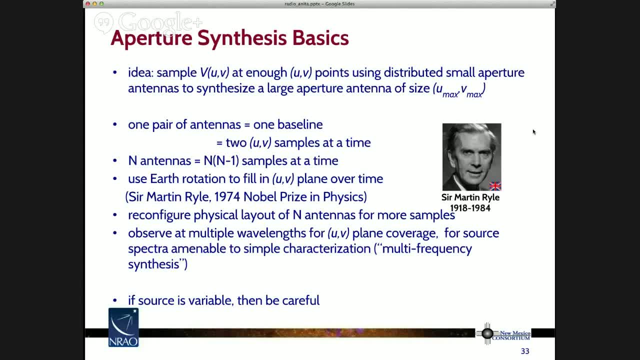 Now, if your source is varying while you're making different measurements of UNV, of visibility, then you're in trouble in terms of aperture synthesis. So one of the assumptions is that while you're collecting all these samples of the Fourier transform, the source isn't changing. 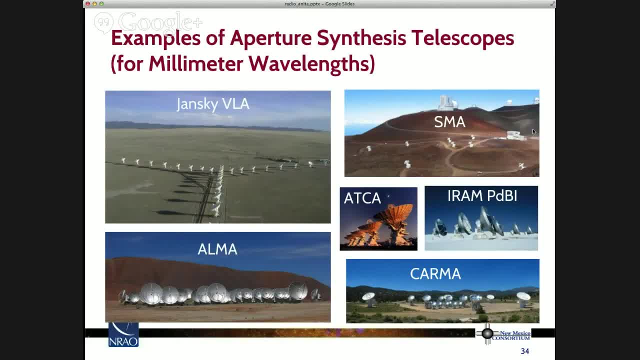 Here are a few examples of aperture synthesis telescopes, in particular ones that work at millimeter wavelengths. I already showed you the VLA and ALMA. here on the left. One of my favorite telescopes is the submillimeter array that our institution helped build. 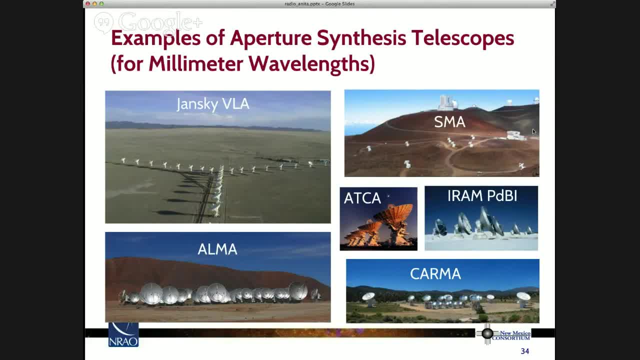 upon Mauna Kea. The Australia Telescope Compact Array is a synthesis telescope, the IRM Plateau-de-Bure Interferometer and the CARMA array in California. You can see, they're all different configurations of multiple antennas, all of which can be moved around. 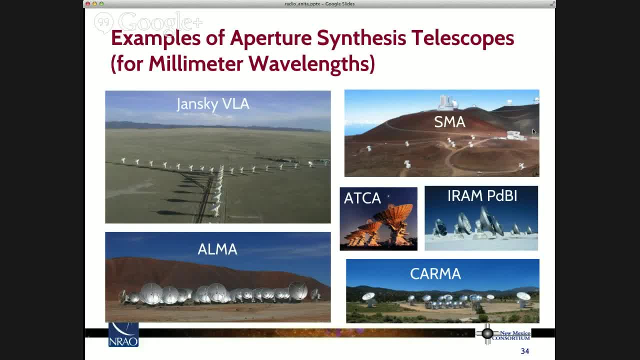 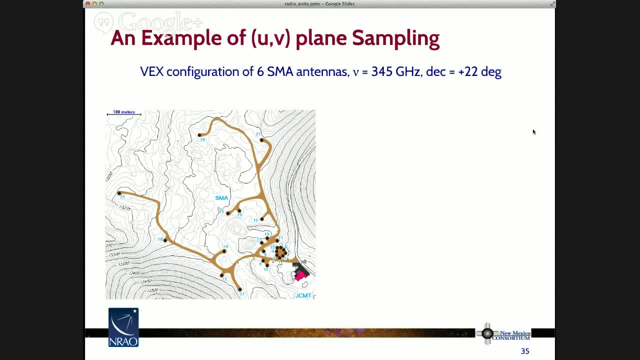 to collect visibilities and ultimately to make images of celestial objects. Alright, So let me give you a concrete example of UV sampling. This is from the submillimeter array. So this picture here on the left are the 24 stations that one can put, each of the 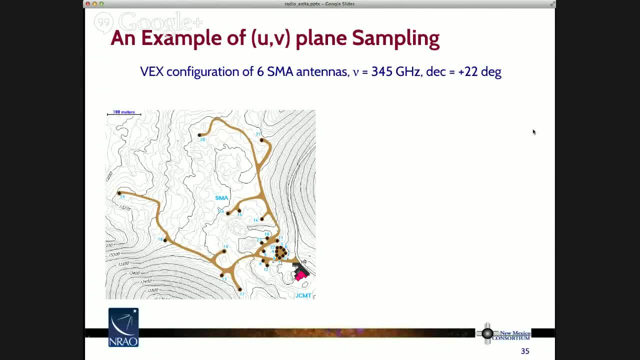 8 antennas of the SMA- In this case we're only using 6 of them- at a frequency of 345 GHz, at a declination of 22 degrees, And we put those 6 antennas in those places and if we let the Earth turn, 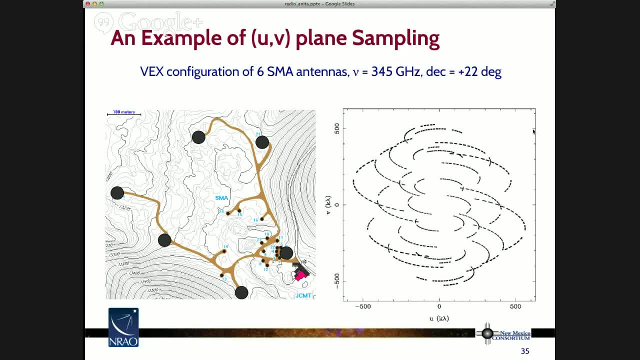 then this is the sampling of the UV plane that one gets out of this particular configuration source at this frequency. So you can see, the span is about a thousand kilolambda, a thousand wavelengths, and in both U and V. and what else to say about this? 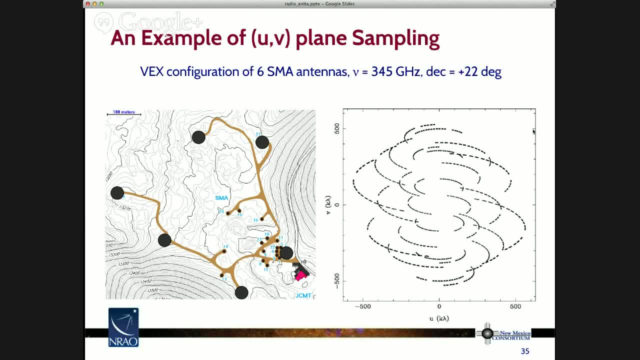 there are lots of little gaps in these elliptical tracks. that's when you're not looking at the target source of interest but you're looking at a calibrator, and there are some longer gaps. maybe when something went wrong, You could then move the antennas around. so here's 7 antennas. 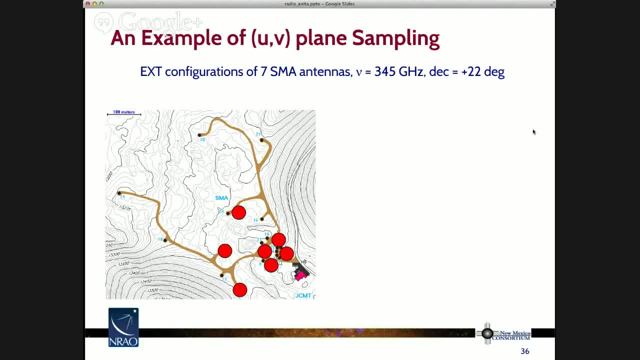 of the array at different stations and the UV coverage looks like this. so now the antennas are closer together, so U and V are smaller. and then here's another configuration: 7 antennas move into an even more compact configuration and that's the coverage you get out of that. 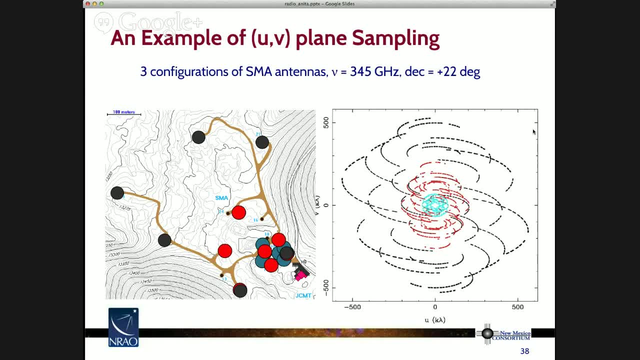 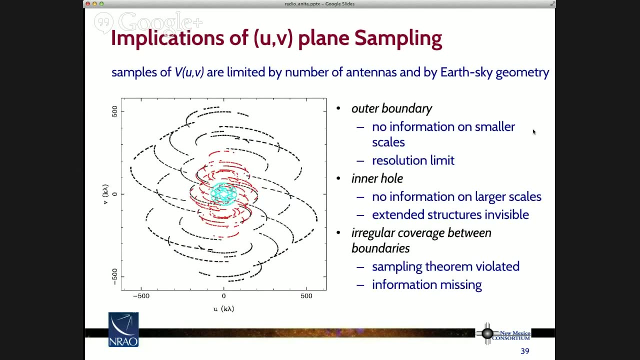 and then you can combine them all and these 3 observations, each of which runs for some 8 hours, gives you this coverage of the UV plane. so all of these different samples of the Fourier transform of the source that we're interested in. So what are the implications? 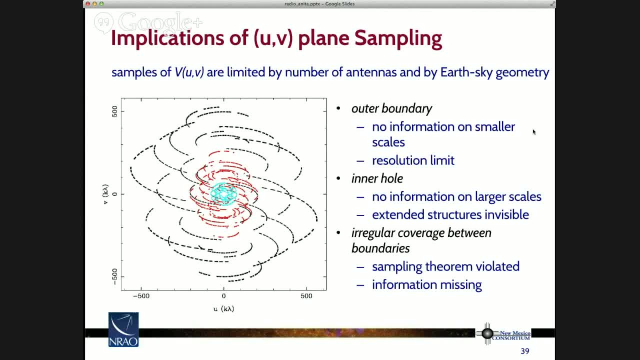 of this kind of coverage. The samples of the visibility function are limited entirely by the number of antennas you're using and by the geometry of the Earth and the target position in the sky. So one typically has a UV coverage like this in the sense that 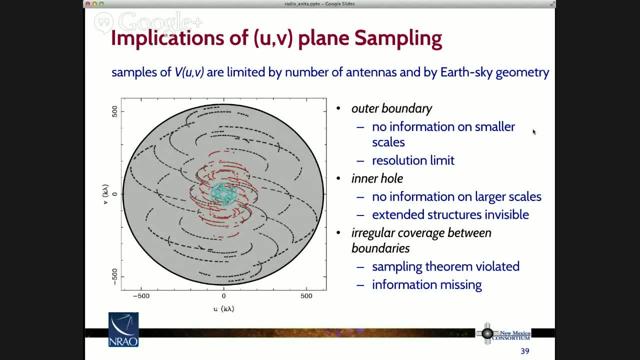 these properties are. there's an outer boundary, so there's no information on size scales that are smaller than what's sampled by the outer boundary. so this corresponds to the resolution limit. so this is the size of our telescope: it's 500,000 wavelengths in every direction. 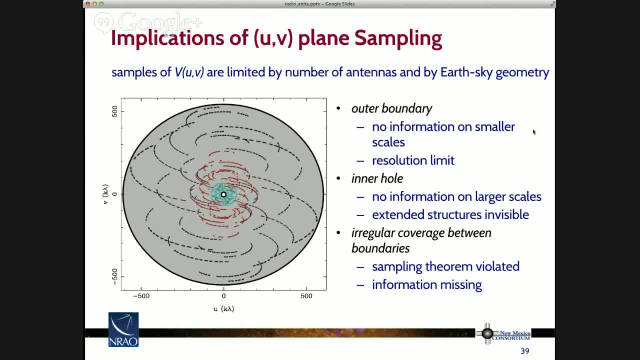 interferometry also usually ends up with an inner hole right in the center there of the UV coverage that you can only put the antennas so close together. so that means there's no information on larger scales than that, and extended structures that are too big are completely invisible. 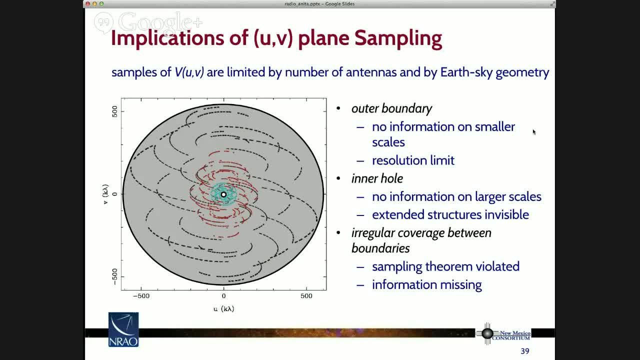 that's not something that we tend to have a lot of intuition about, but it's a very important feature. and then, in between this inner hole and the outer boundary, we have irregular coverage based on where we could put the antennas and how the Earth was rotating and where the source was in the sky. 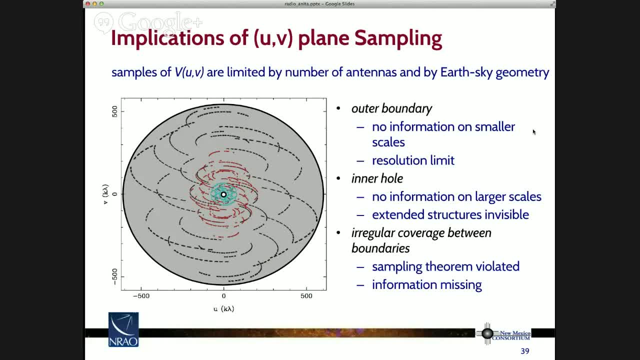 and so typically the sampling theorem is violated and information is missing. so all this sounds terrible, but it's not so bad, and the imaging and deconvolution lecture will talk about how you can recover from some of these problems, just to give you a little more intuition about these two issues. 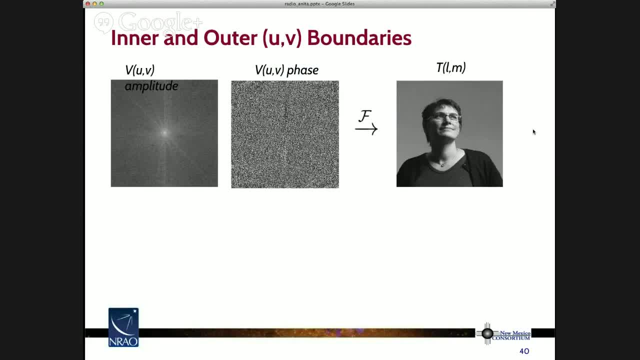 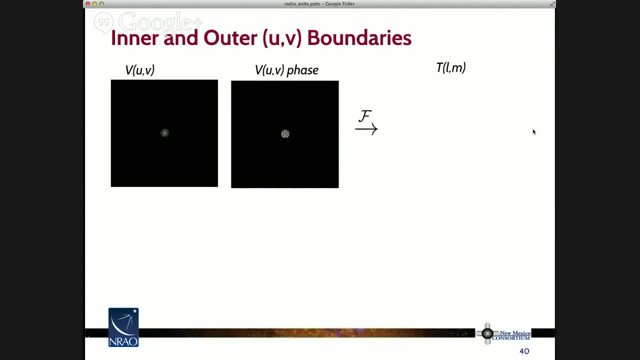 here is our Fourier transform of an astronomer. again, remember the amplitude and phase. if we were to get rid of all the high spatial frequencies, just apply this mask, and so we only measured the ones in the middle there. then we just get a blurry version of the astronomer. 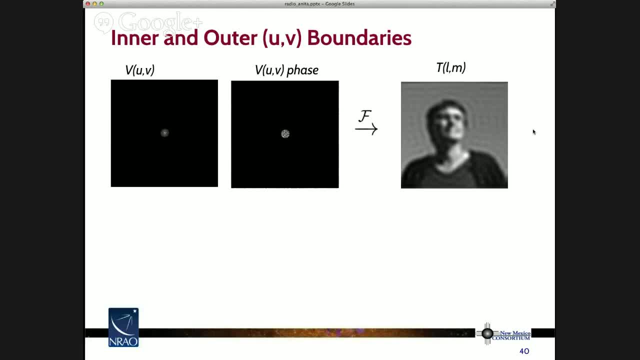 right. our resolution is limited. so just like observing with a small telescope instead of a big one, or with your eyeball instead of the Hubble space telescope, things are blurrier. but the opposite is also true if we were to lose the low spatial frequencies, the ones in the middle, 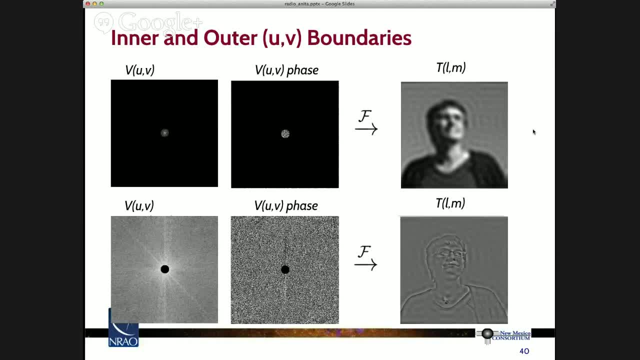 the Fourier transform of that is a highly spatially filtered version of the astronomer. we only see the edges. the total flux is gone because that was in the middle total flux density gone. but you pick up all the small scale features. so maybe, like the smiley face in my 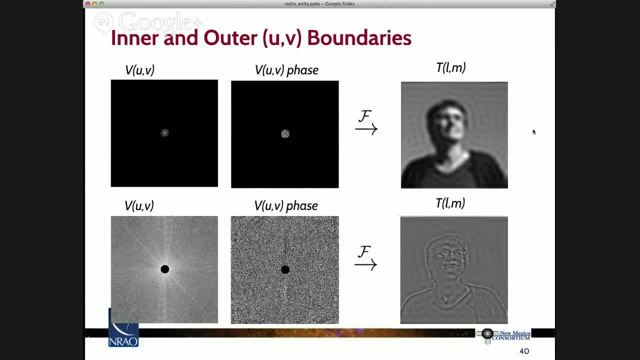 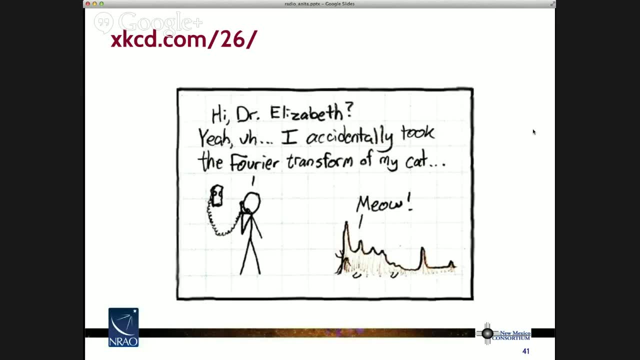 example, but in this case an astronomer's smiley face. so Fourier transforms are great. they're fundamental to interferometry, and if you're not familiar with XKCD- I hope you will be- you can take a look at this cartoon at your leisure. but if you 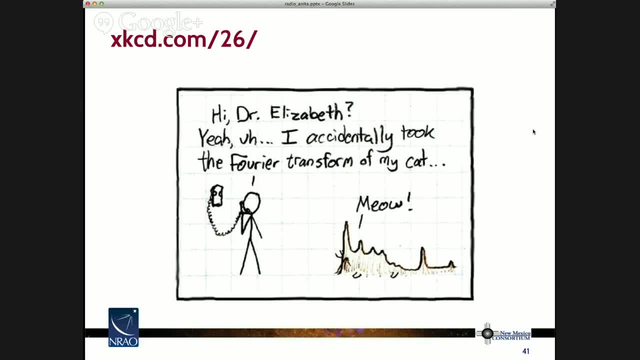 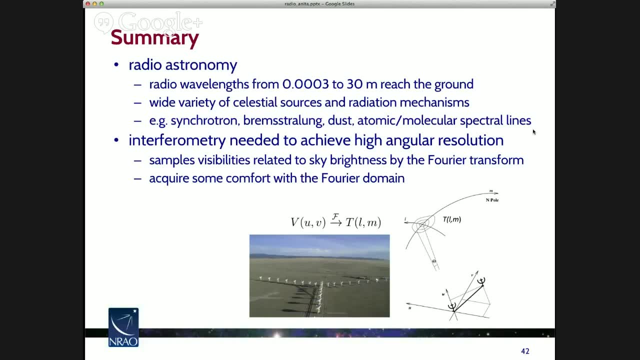 accidentally, Fourier, transform your cat. you're in trouble. and to summarize, what have I talked about today? I've talked a little bit about radio astronomy. the things to remember are that radio wavelengths from a few hundred microns to tens of meters reach the ground. there are many different kinds of celestial sources. 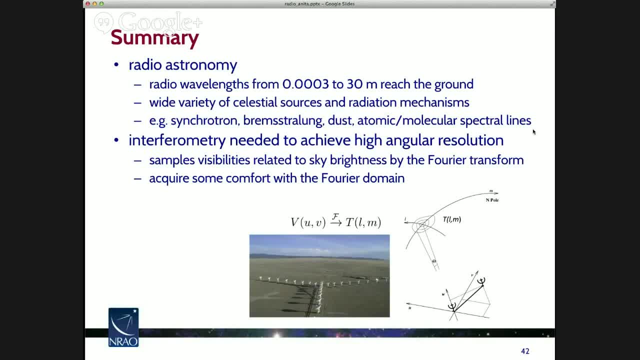 and radiation mechanisms in this wavelength range, including, I described, synchrotron Armstrong, dust emission, atomic and molecular spectral lines, and all these get windows on the universe that are not available, say in the optical, which is the only other wavelength regime that reaches the ground, and, if you want high angular resolution,